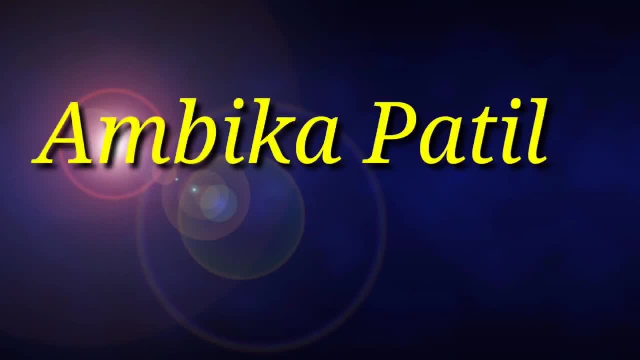 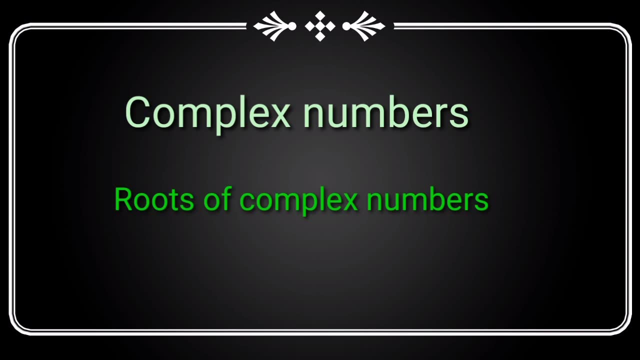 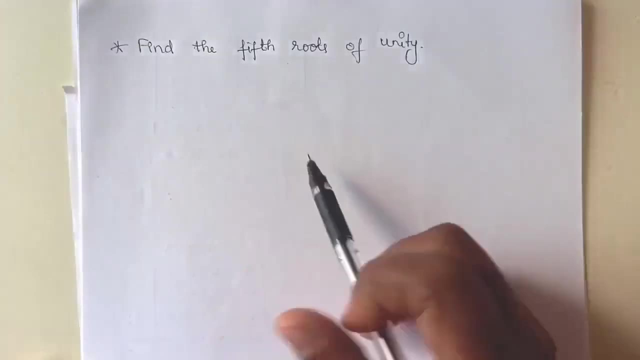 Hello students, welcome back to my channel. In the last class we have discussed about how to find the roots of the complex number. So here we have few more examples on the roots of the complex number. So next problem is find the 5th root of unity. 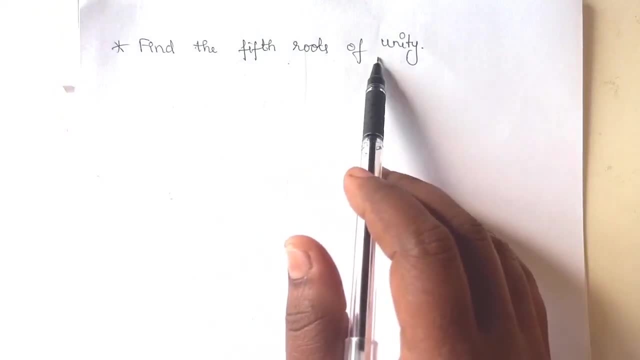 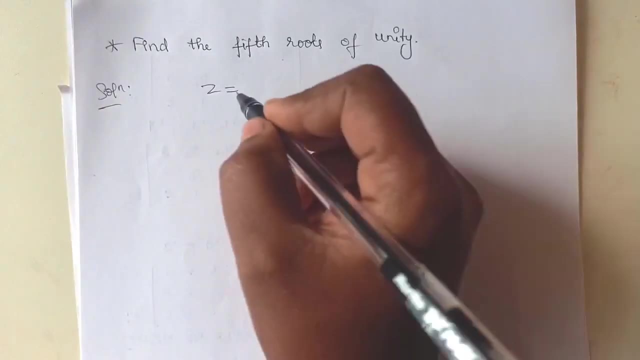 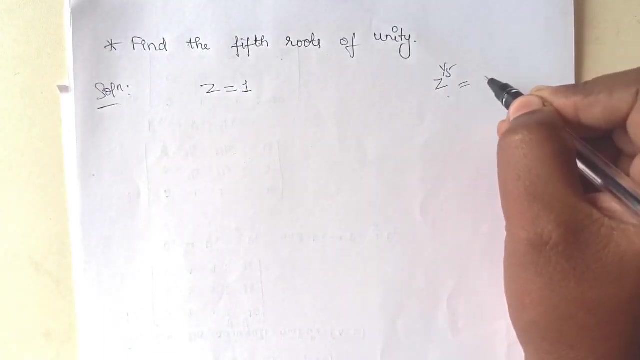 So here, given that the question is: find the 5th root of unity, Unity means 1.. So that here, given complex number is z equals to unity means 1.. Now we want to find out the 5th root of this complex number, that is, 5th root of this complex. 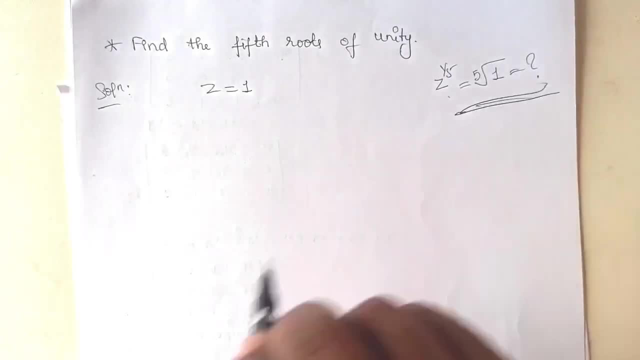 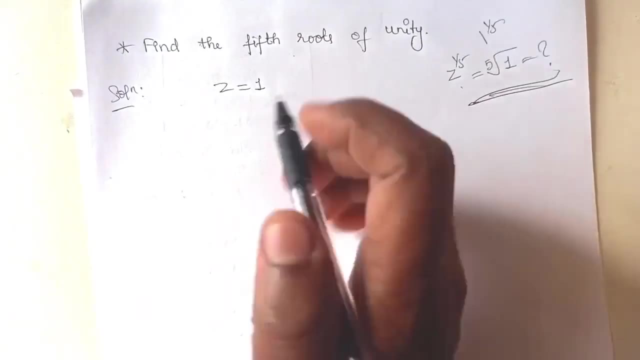 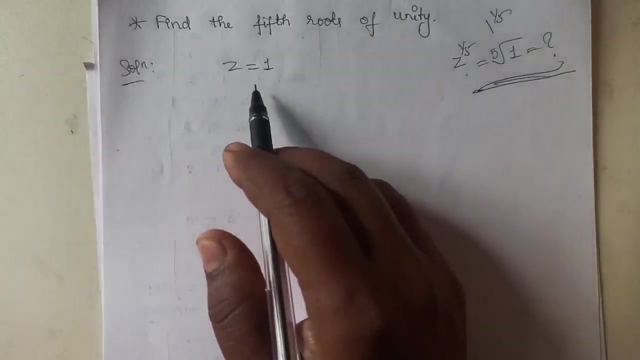 number This 1.. Now we want to calculate this one or 1 power, 1 by 5.. So for this we start with finding r and theta value. So here z equals to 1.. So that means, given complex number, is z equals to 1.. 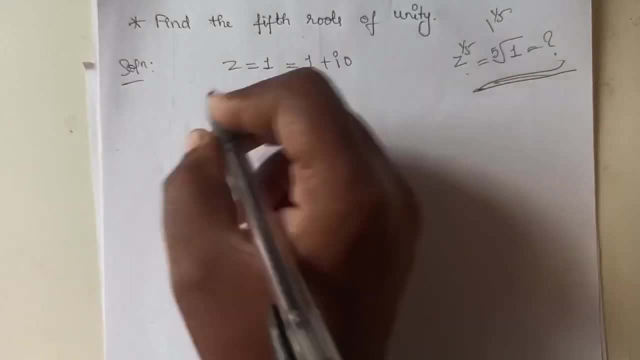 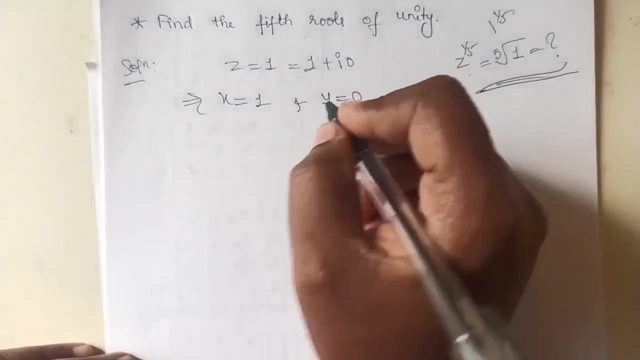 This can be written as 1 plus i into 0. That means x is equals to 1.. And y is equal to 0. So that r value is equal to square root of x square plus y square is 1 plus 0, which is: 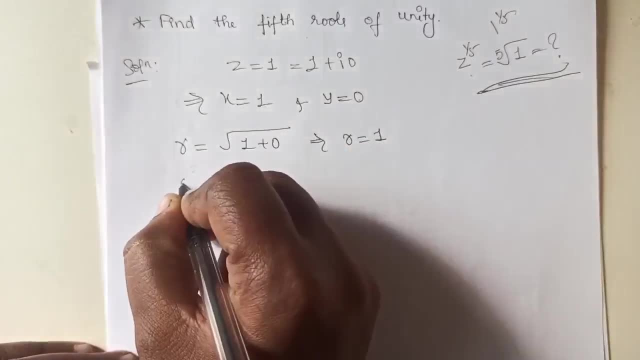 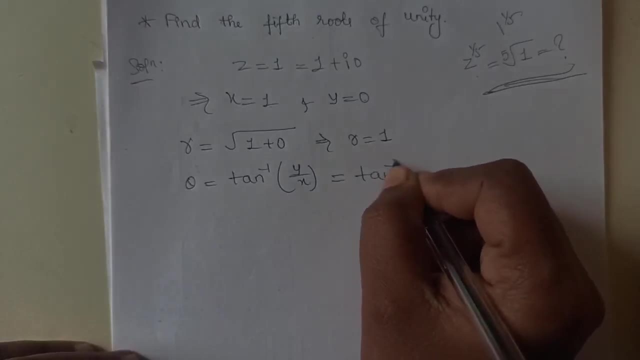 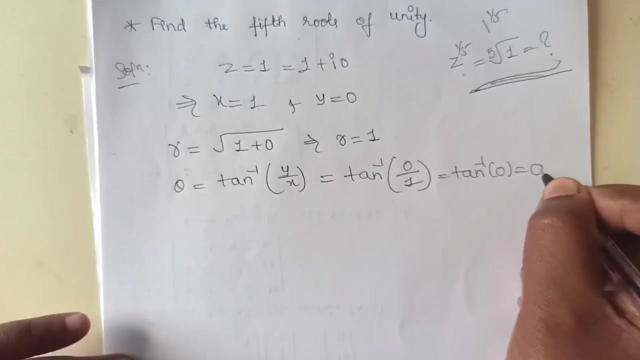 equal to r, value equals to 1.. And theta is equal to tan inverse of y by x. So that is, tan inverse of y value is 0 by 1, which is equal to tan inverse of 0, which is equal to 0.. 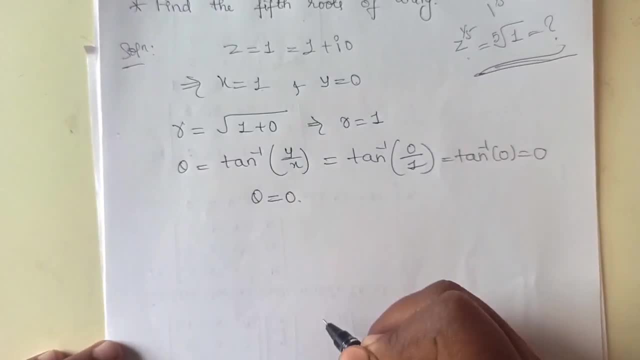 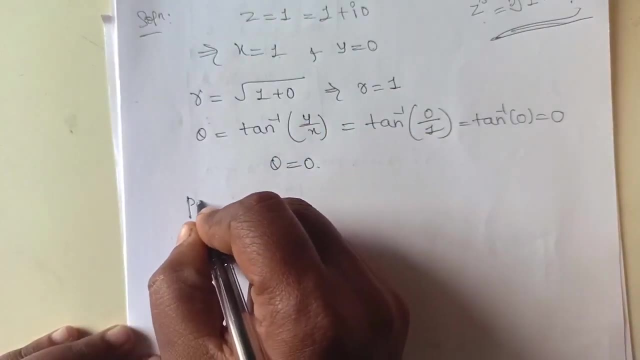 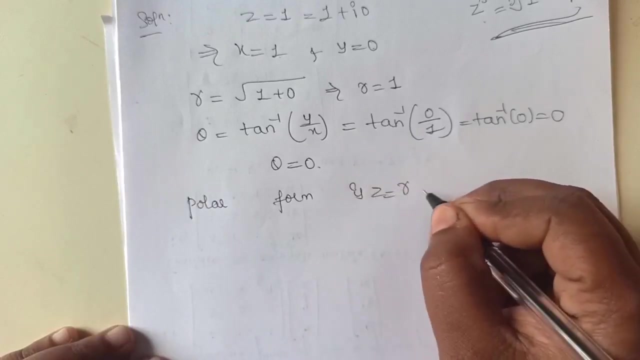 So that theta value is equal to 0.. So that z equals to 1.. So we have seen r is equal to 1.. Now we want to represent it in terms of polar form. that is, the polar form is r is equals to, so that z is equal to r into cos theta plus i sine theta. 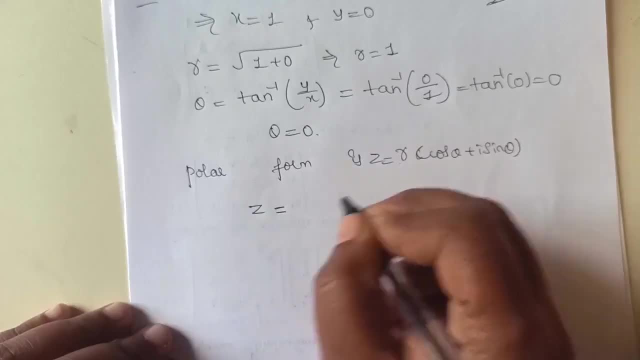 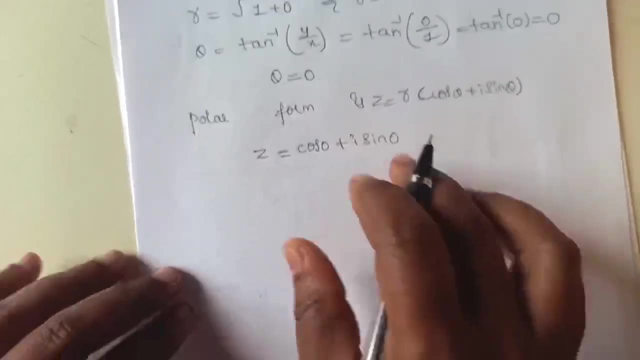 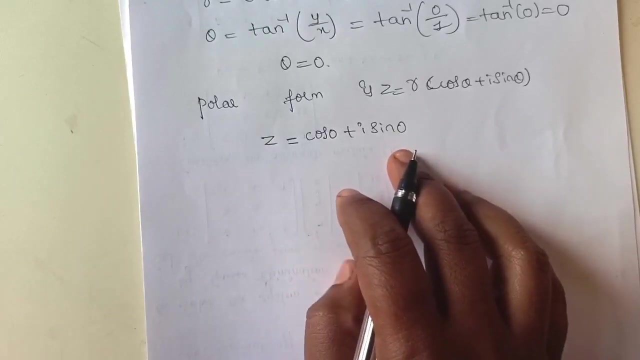 Here z equals to r value is 1.. Therefore we get cos of 0 plus i sine 0.. 0.. Right Now we replace this 0 by 2n pi plus theta. Okay, So the next step is replace theta. 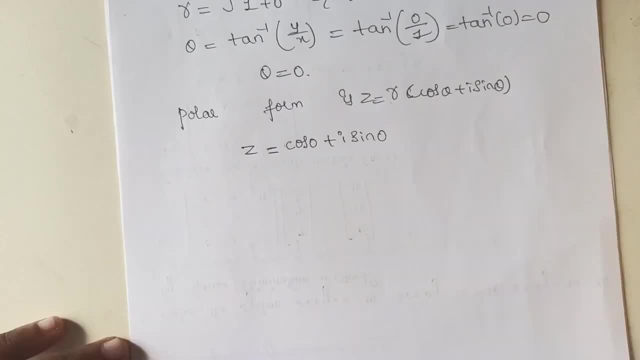 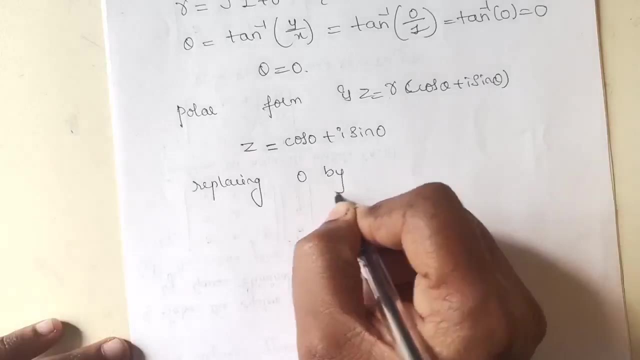 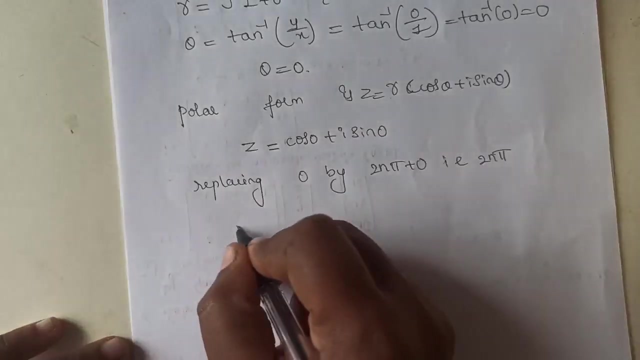 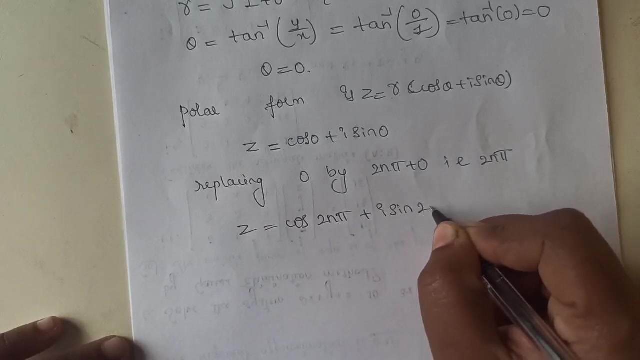 by 2n pi plus theta. Replacing 0 by 2n pi plus 0, that is 2n pi, we get z becomes cos of 2n pi plus i sin 2n pi. Okay, Consider so this equation is okay. We consider this. 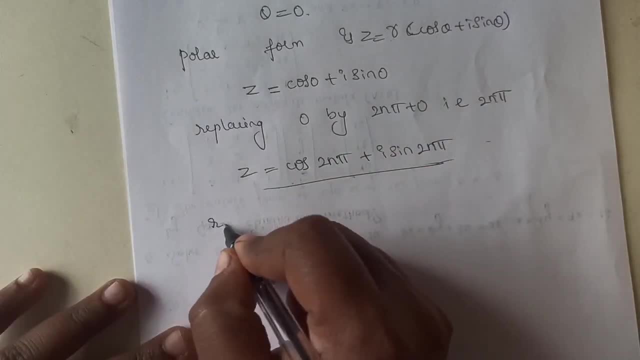 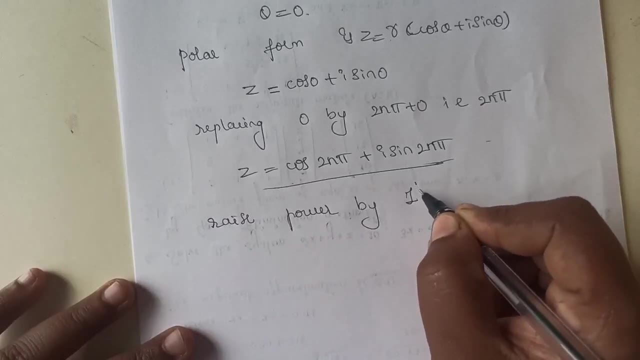 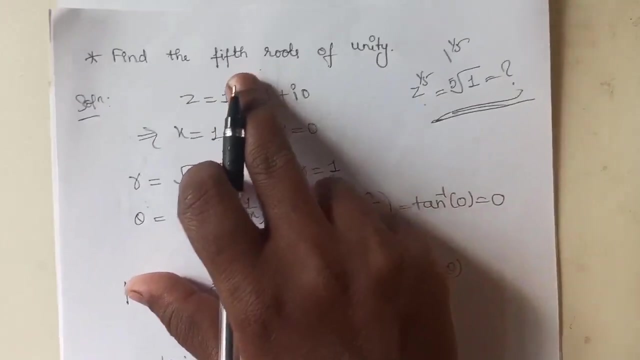 as equation 1: or we raise the power on both side. raise power by 1 by 5 on both side. Why we raise 1 by 5?? Since we want to find fifth root of unity, that is, z power 1 by 5.. Okay, 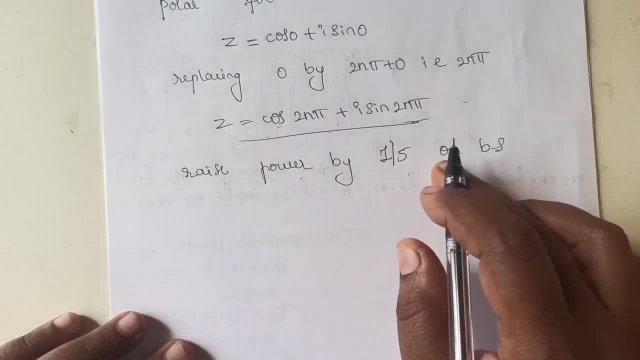 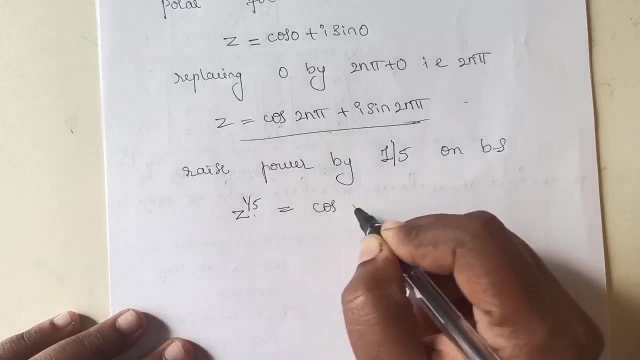 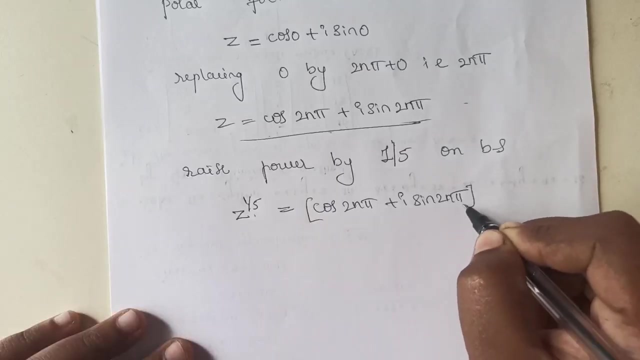 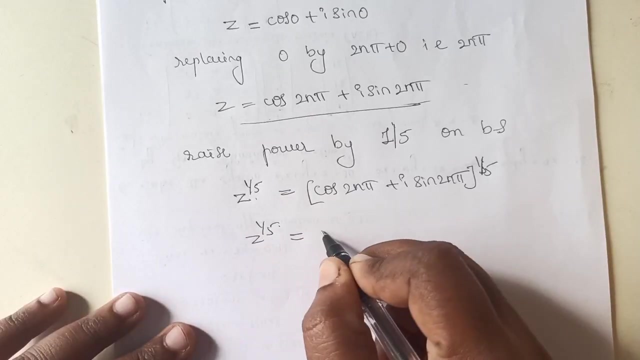 Therefore we raise the power 1 by 5. on both sides Raising power we get z power 1 by 5 equals to cos 2n pi plus i sin 2n pi power 1 by 5.. So, applying DeMurray's theorem, this can be written as z power 1 by 5 cos. 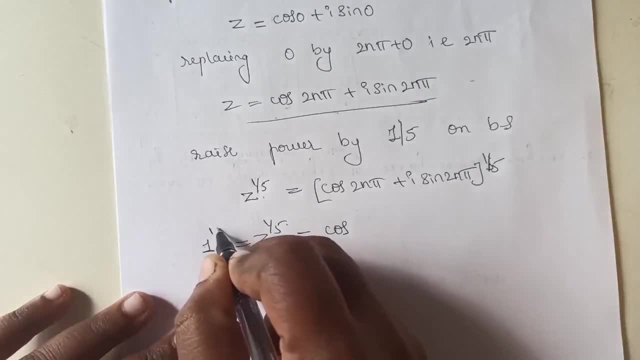 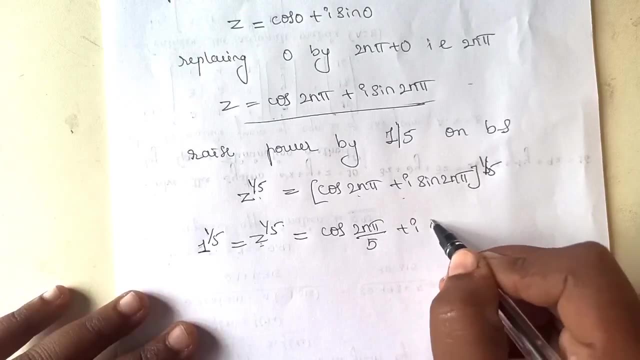 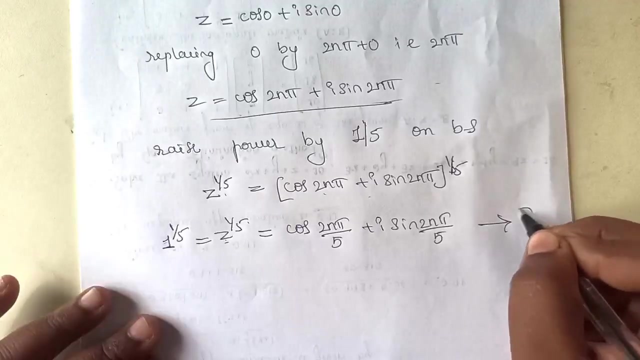 So z means it is given complex number which is 1 power 1 by 5.. Is equals to cos 2n pi by 5 plus i. sin 2n pi plus i mean divided by 5.. So consider this as equation 1, and this one is very, very important for the calculation. 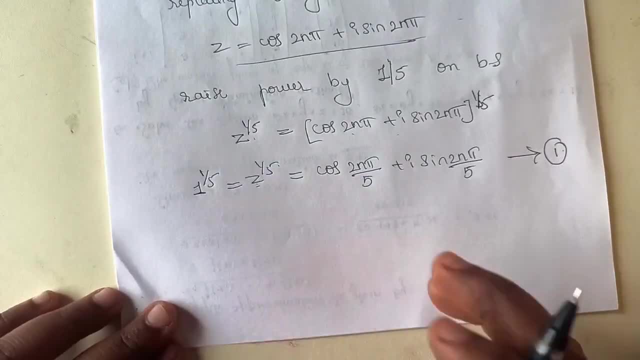 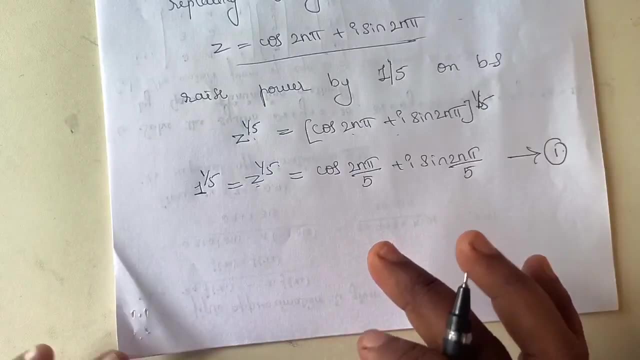 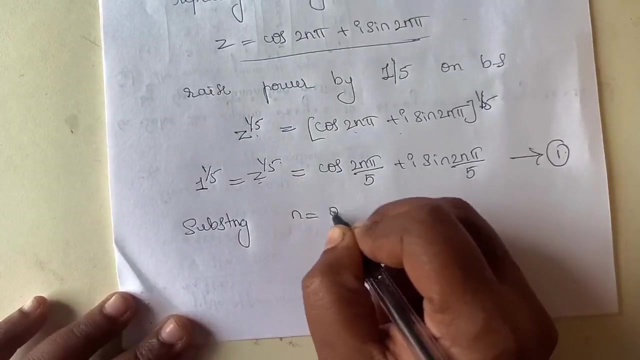 So now we substitute n equals to 0, n equals to 1, up to n equals to 4.. Since we want 5th root, therefore, we substitute n equals to 0 to 4.. Okay, Now, substituting n equals to 0,, 1,, 2,, 3,, 4 in 1, we get. 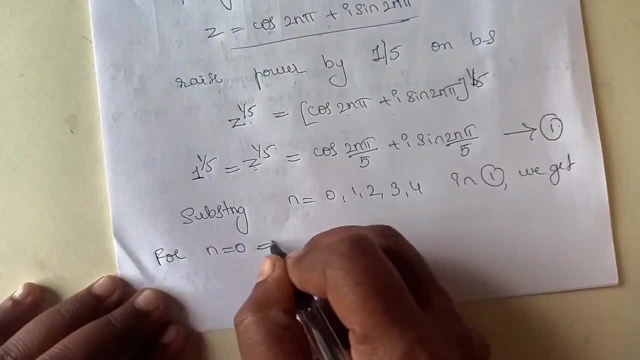 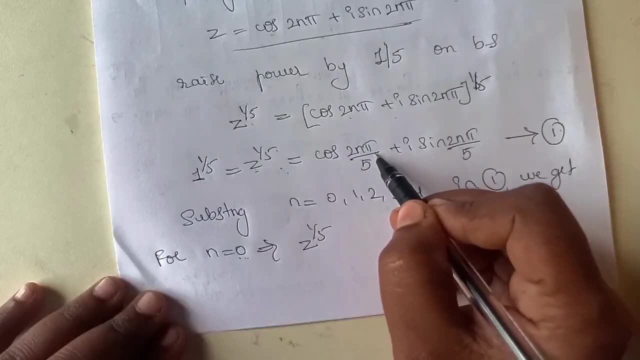 So for n equals to 0, we get this equation: 1 becomes z power 1 by 5.. Now substituting n equals to 0, here this term becomes 0.. Totally 0.. That is cos of 0 plus i sin 0. 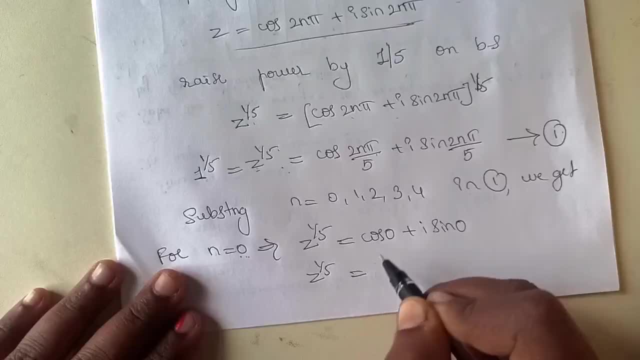 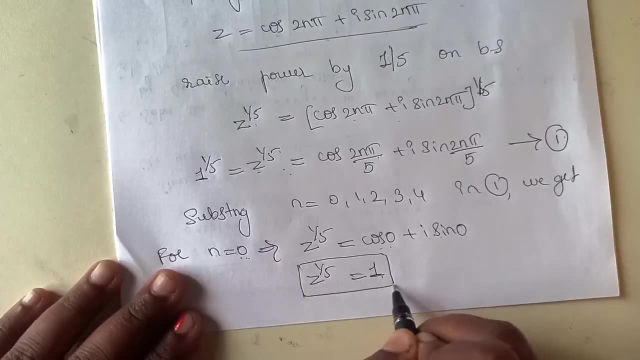 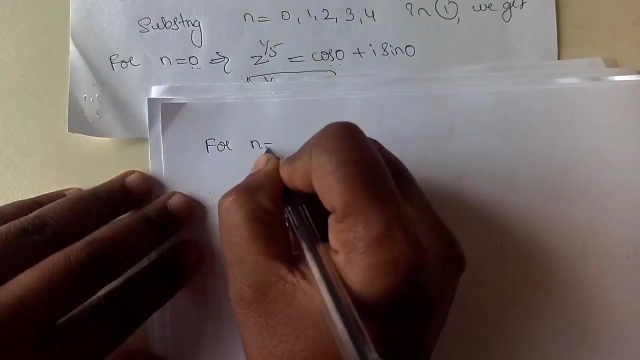 So we get the first root is: cos of 0 equals to 1, plus i sin 0 equals to 0. Therefore we get 1.. So this is the first root. Okay Now for n equals to 1, equation 1 becomes z power 1 by 5.. 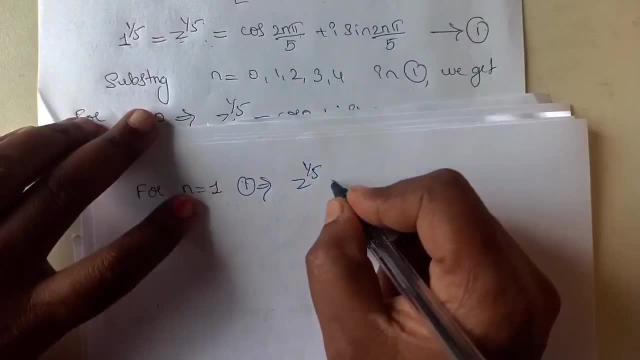 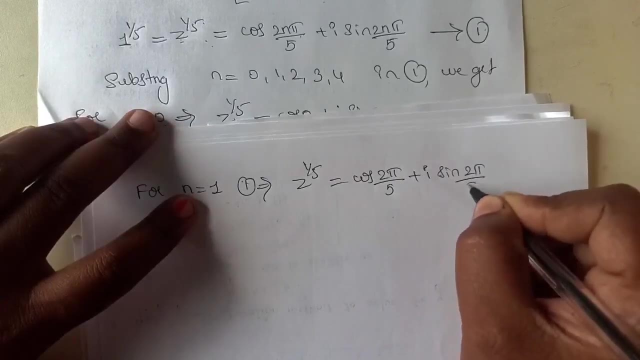 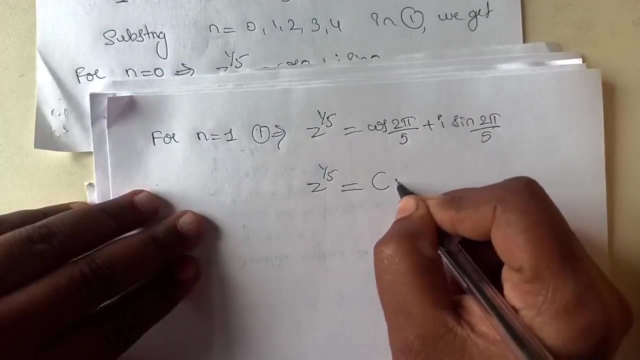 So substituting n equals to 1, it becomes 2 pi by 5.. So cos of 2 pi by 5.. So this can be written as z power 1 by 5.. Cos plus i sin can be written as cis. 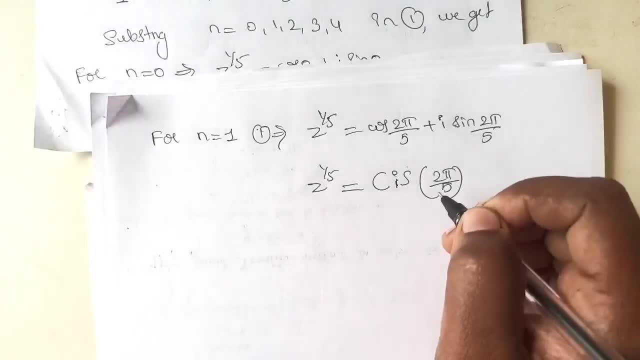 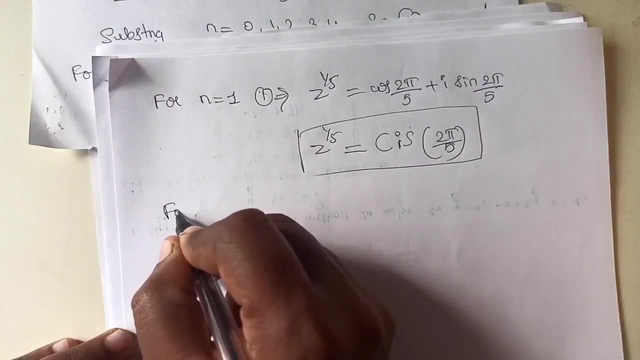 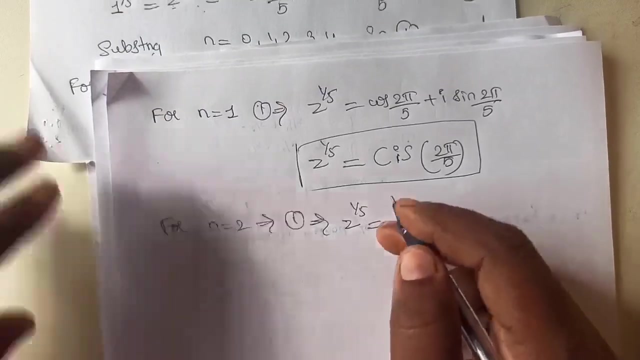 Okay, Cis of 2 pi by 5.. Okay, So therefore this is the second root. Similarly, for n equals to 2, equation 1 becomes z power 1 by 5.. So substituting n equals to 2.. 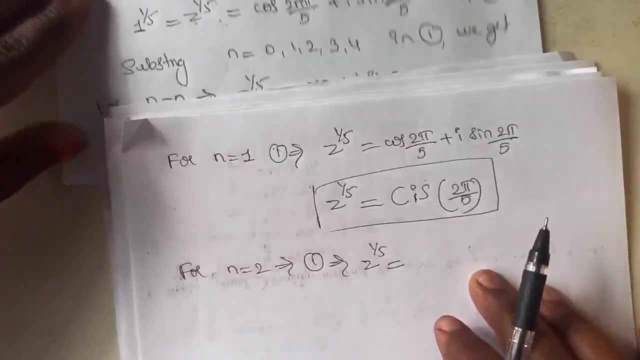 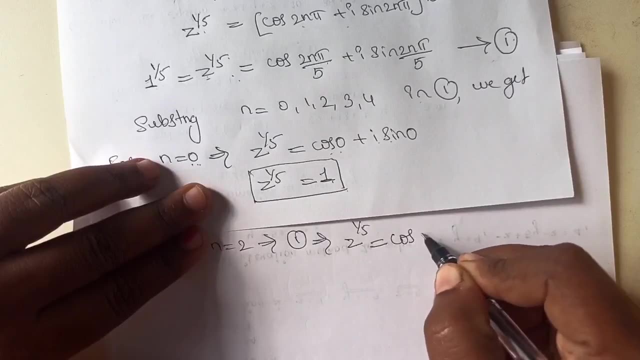 Here, 2 into 2 is equals to 4, 4 pi by 5.. Okay, So substituting n equals to 2 in equation 1, we get cos of 4 pi by 5, plus i sin 4 pi by 5.. 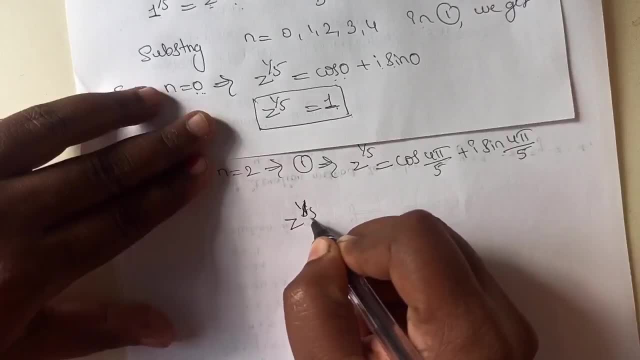 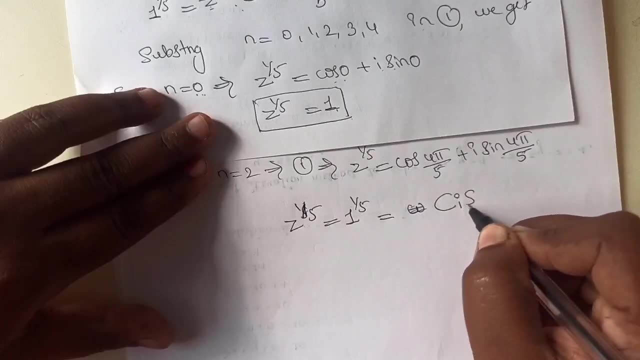 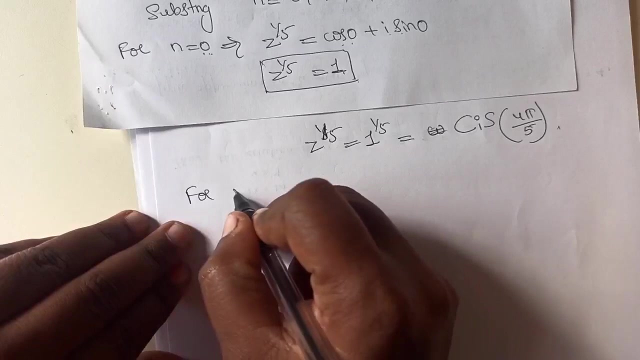 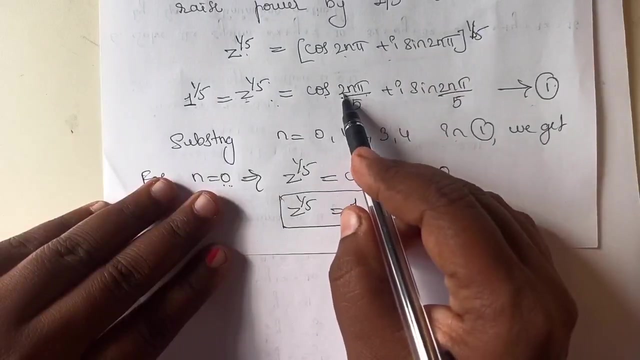 So that the second root, that is 1 power, 1 by 5, is. this can be written as cis 4 pi by 5.. So next, for n equals to 3, equation 1 becomes. so substituting n equals to 3, it becomes 2 into 3 is equals to 6, 6 pi by 5.. 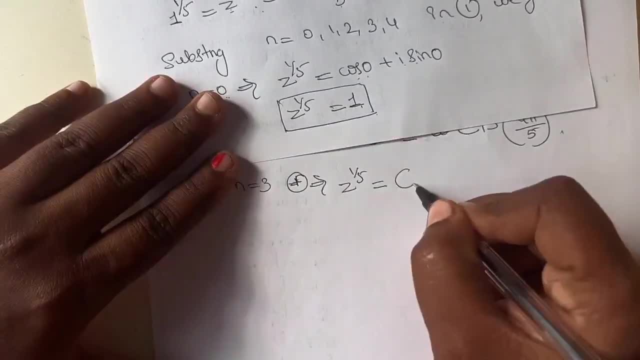 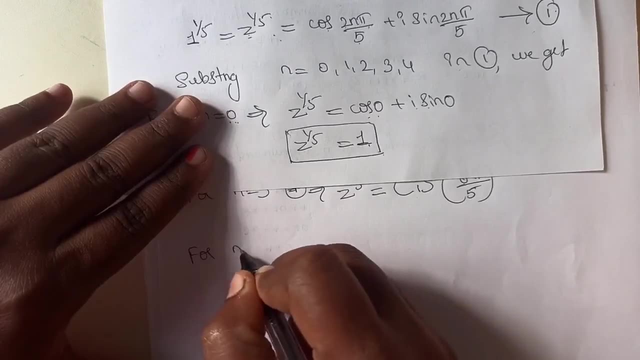 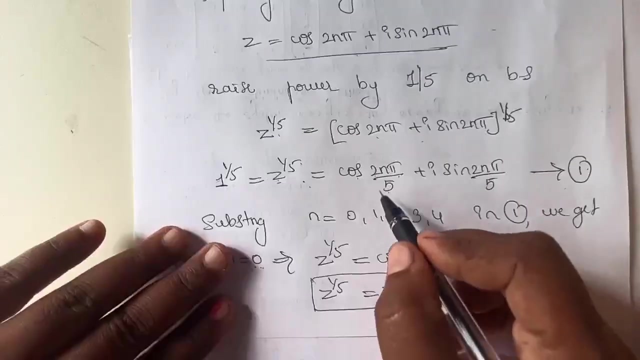 So therefore z power 1 by 5 is cis of 6 pi by 5.. So next, for n equals to 4, equation 1 becomes z power 1 by 5.. So substituting n equals to 4, we get 2 into 4 is equals to 8, 8 pi by 5.. 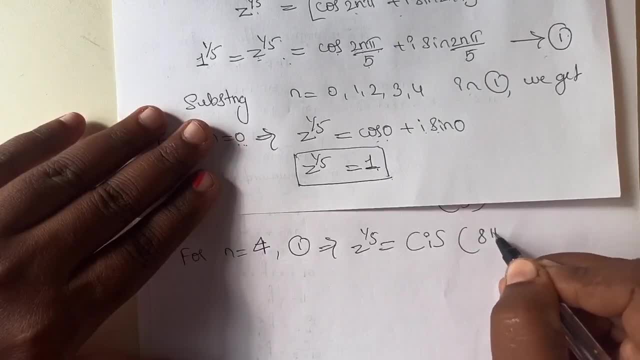 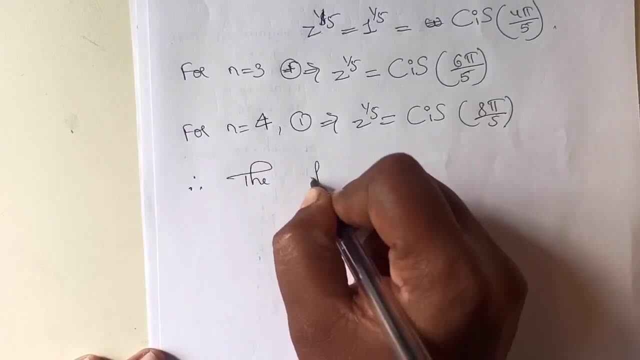 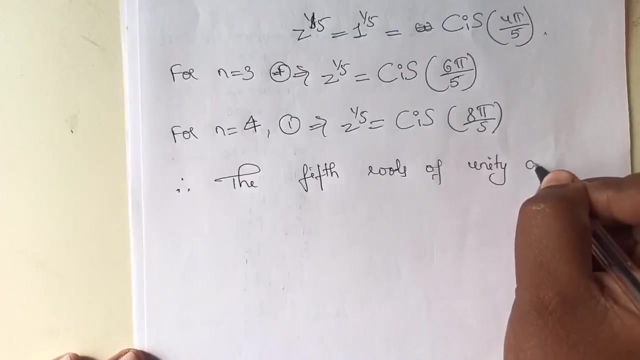 So therefore we get cis 8 pi by 5.. So therefore the fifth roots of unity are: so that is 1 power 1 by 5.. So that is 1 power 1 by 5.. 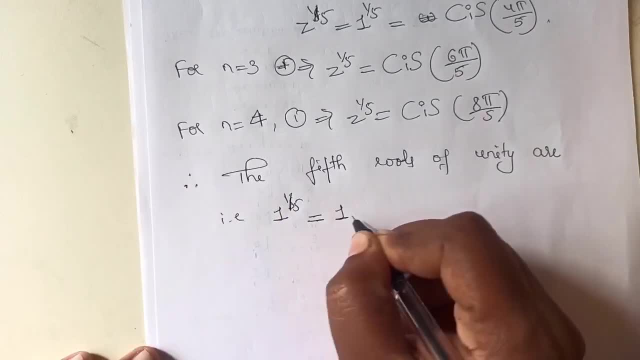 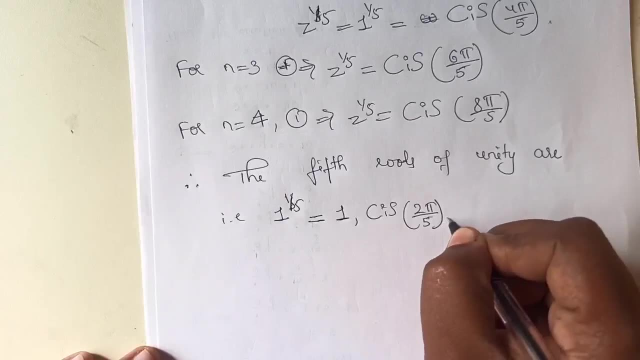 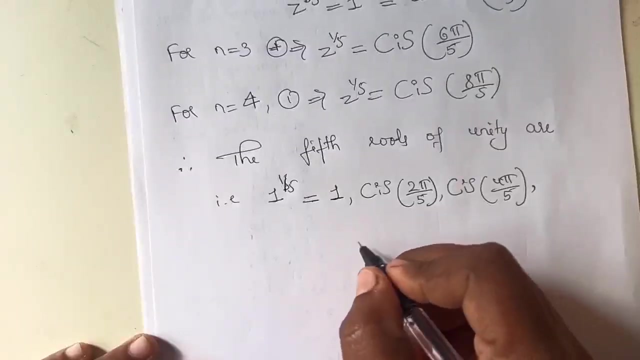 So that is 1 power, 1 by 5.. 5 are: first root is 1, second root is 6, 2 pi by 5,. third is 6, 4 pi by 5, next 6, 6. 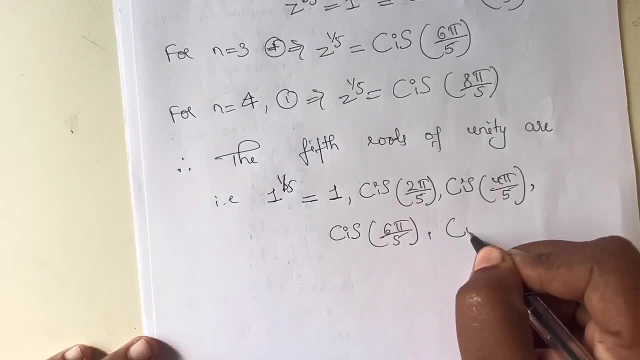 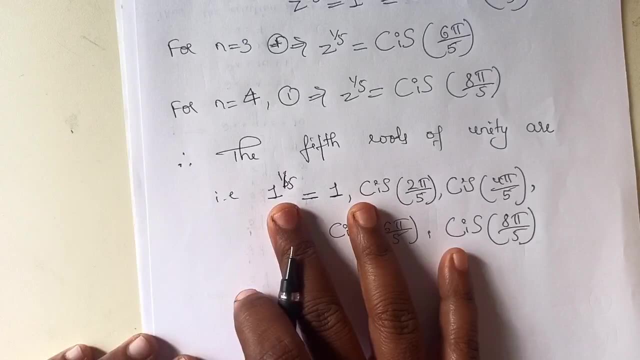 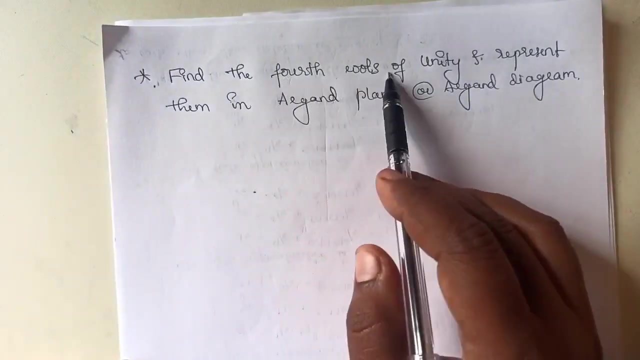 pi by 5, next 6,, 8 pi by 5, so these are the 5 roots of 1,, that is, 5th roots of unity. ok, next problem: find the 4th roots of unity and represent them in the arcane plane or. 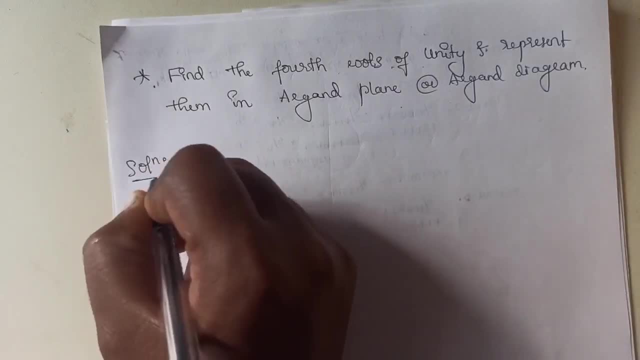 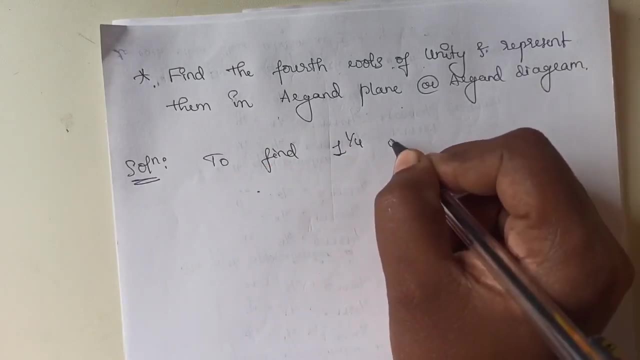 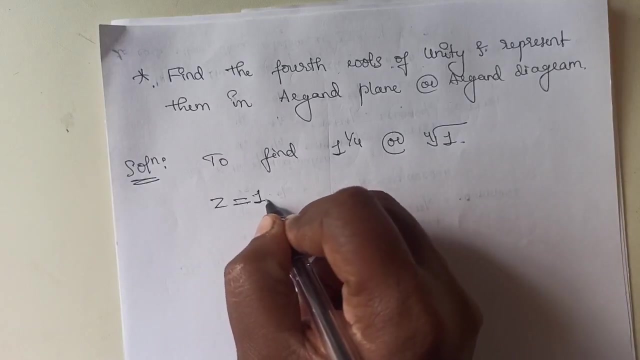 solution. So now we want to find to find 1 power, 1 by 4, or this can be written as 4th roots of 1, so there we consider z equals to 1,, so implies that x equals to 1 and y equals to. 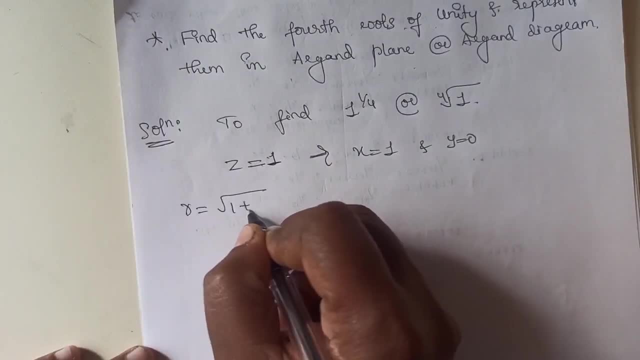 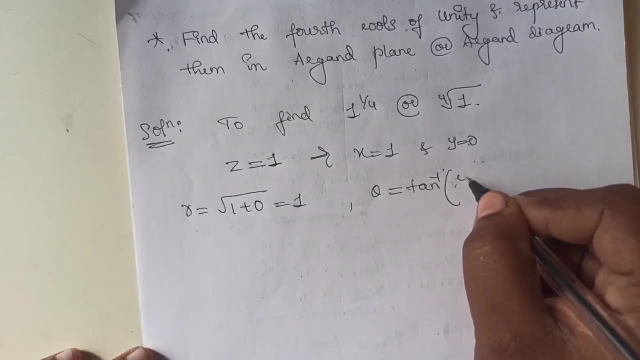 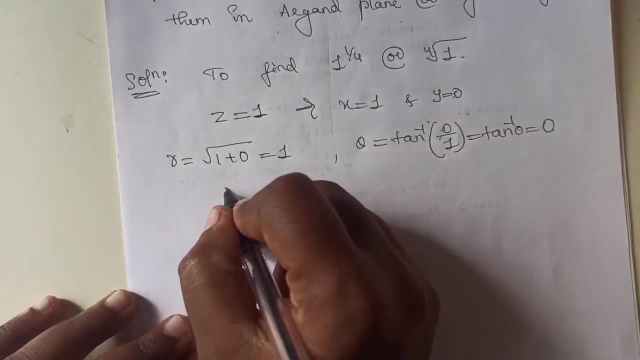 0, therefore our value is: square root of 1 plus 0 is equals to 1 and obviously theta is tan inverse of 1.. So y by x is tan inverse of 0 is equals to 0, ok, so thus r equals to 1 and theta is: 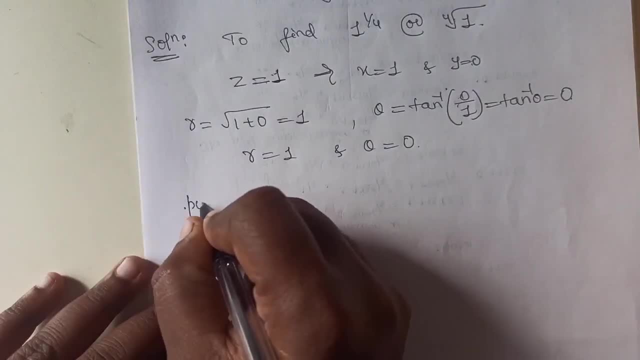 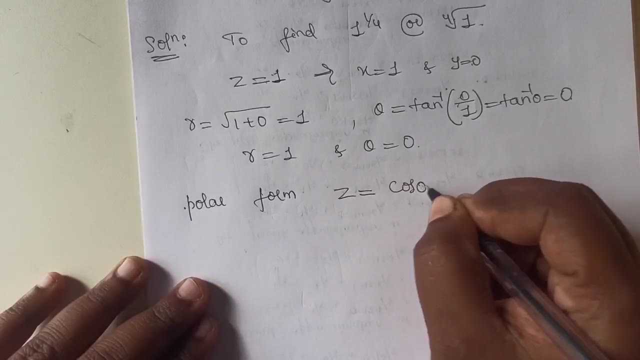 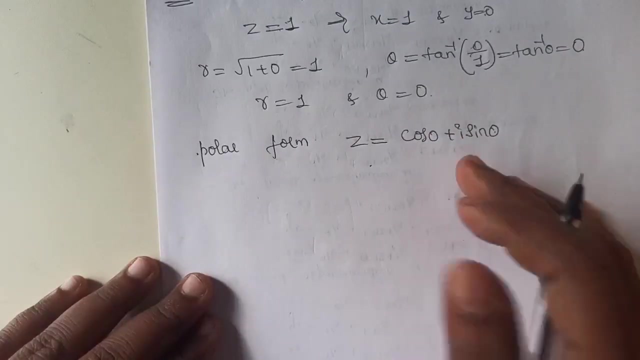 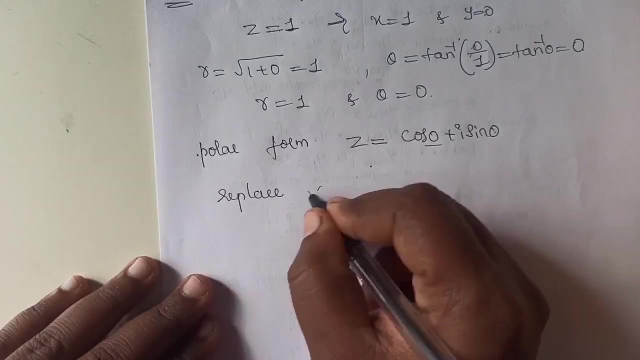 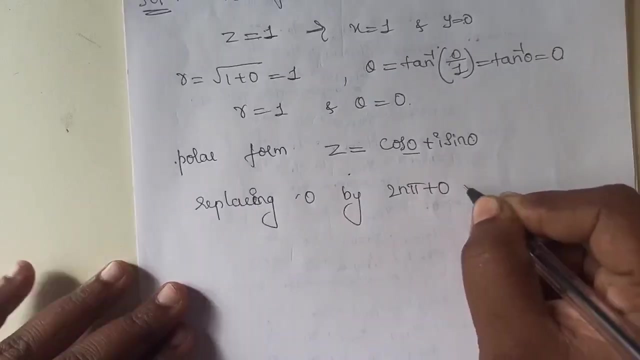 equals to 0. So now, representing in polar form, we get: z is equals to cos 0 plus i sin 0, right, so next we raise power. next We replace this 0 by 2n pi plus 0, so replacing 0 by 2n pi plus 0, which is equals to 2n pi. 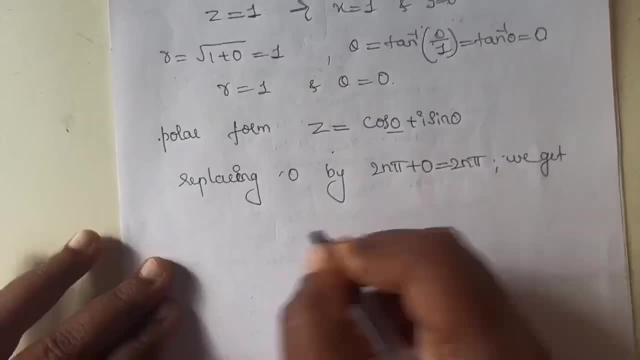 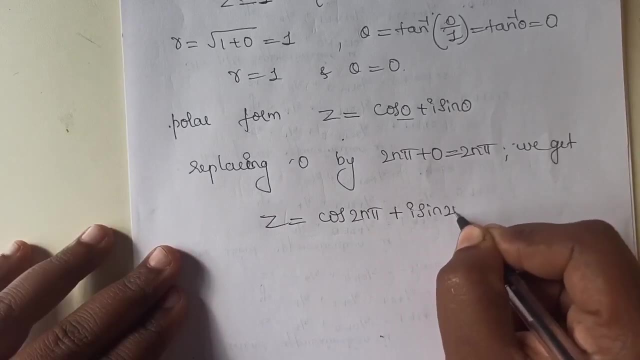 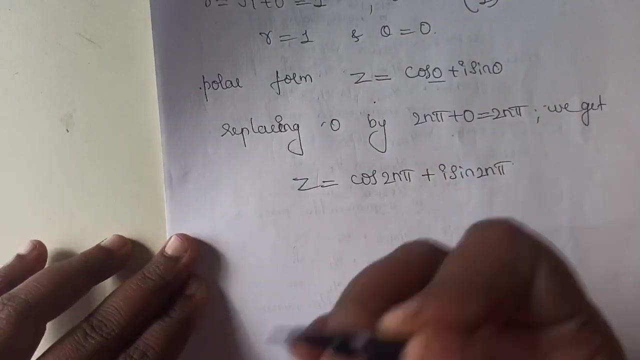 we get z equals to cos 2n pi plus i sin 2n pi. ok, So we want to calculate Fourth root of unity, that is, 1 by 1 power, 1 by 4, therefore we raise. so that is raising. 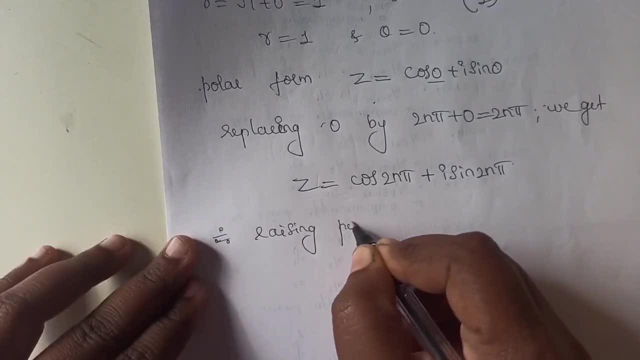 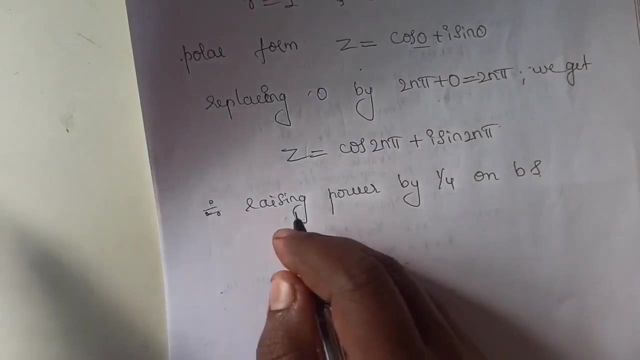 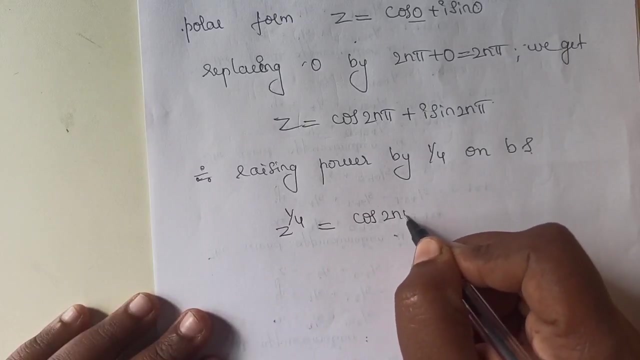 power by 1 by 4 on both side, we get z power 1 by 4 equals to cos 2n pi plus i sin 2n pi. power 1 by 2n pi. So we get z power 1 by 4 equals to cos 2n pi plus i sin 2n pi. power 1 by 4 on both side. 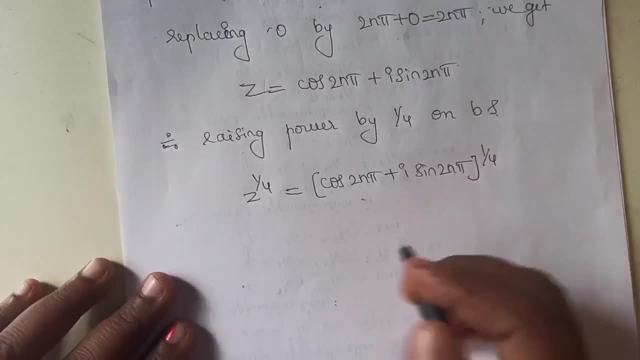 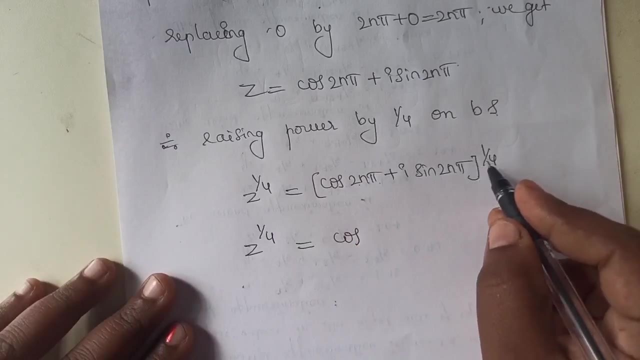 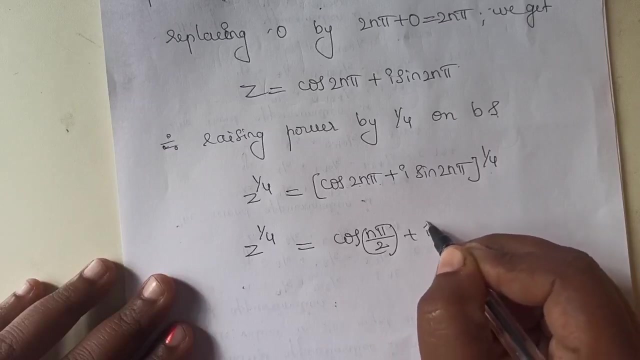 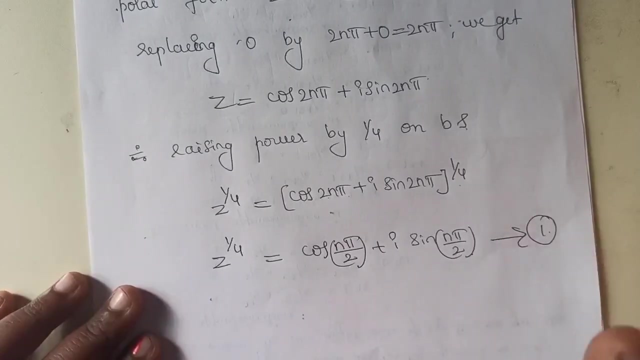 1 by 4.. Now applying de Mouris theorem here, it becomes: z power 1 by 4 equals to cos of 2 n pi by 4, which is equals to n pi by 2 plus i sin n pi by 2.. So this is the required equation Here. 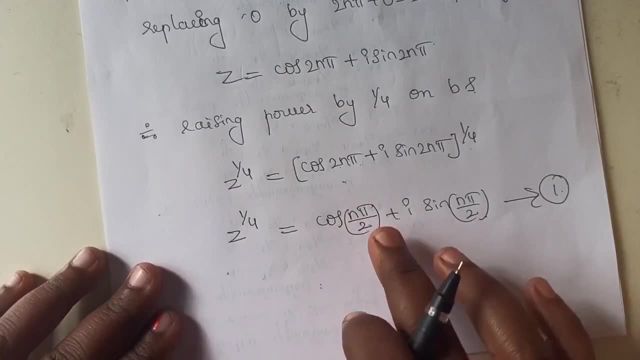 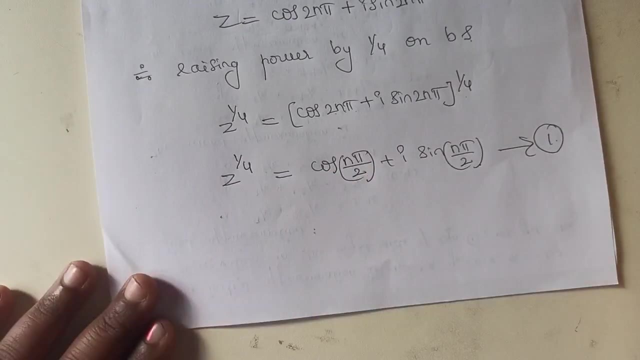 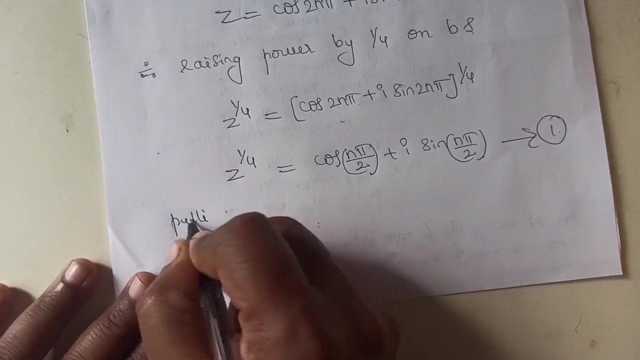 angle is n, pi by 2.. So this angle is called as the argument. Now for 4 roots we need to substitute n equals to 0,, 1,, 2, 3.. Now, substituting n equals to 0,, 1,, 2,, 3 in 1, we get 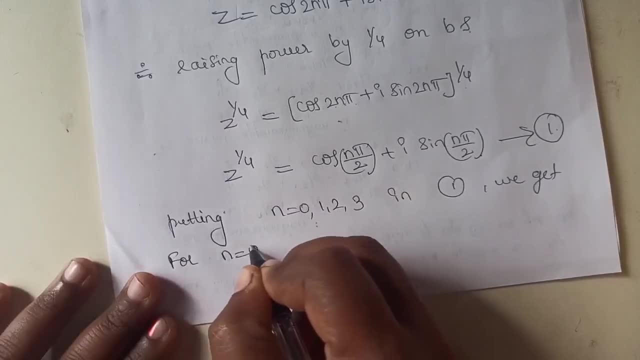 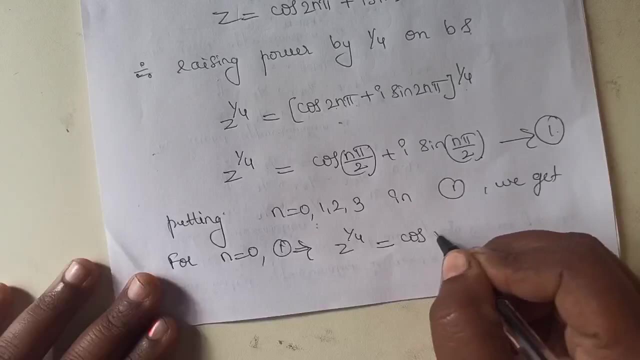 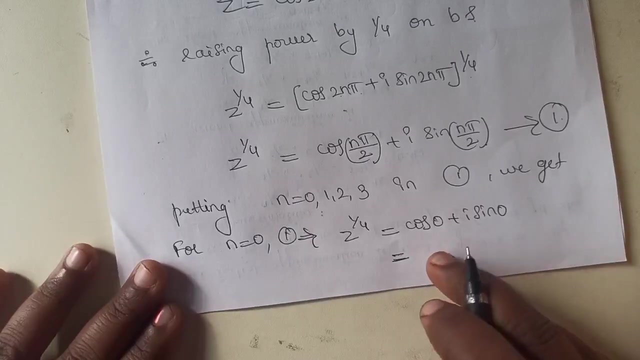 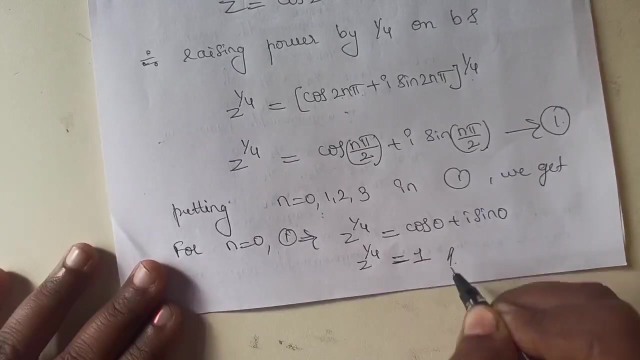 so for n equals to 0, equation 1 becomes z power 1 by 4 equals to cos of 0 plus i sin 0. So substituting this so we get cos of 0 plus i sin 0, that is z power 1 by 4 equals to 1.. This is the first root. 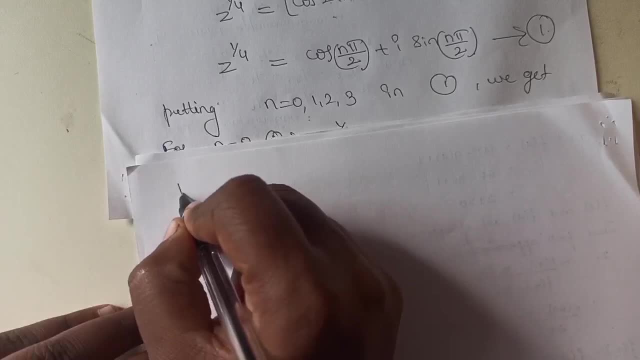 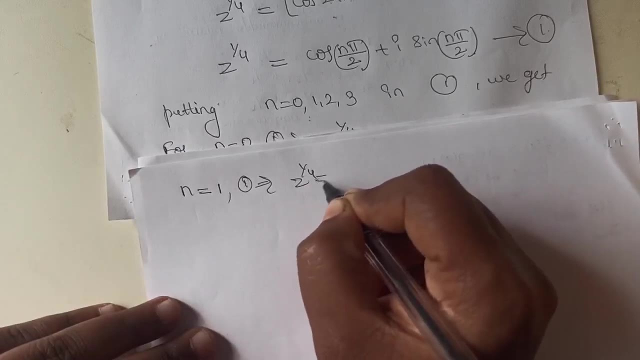 Next, for n equals to 1, equation 1 becomes z power 1 by 4 equals to 1.. So substituting this, we get cos of 0 plus i sin 0. Equation 1 implies that z power 1 by 4.. So here, substituting n equals to 1, we get cos pi by 2. 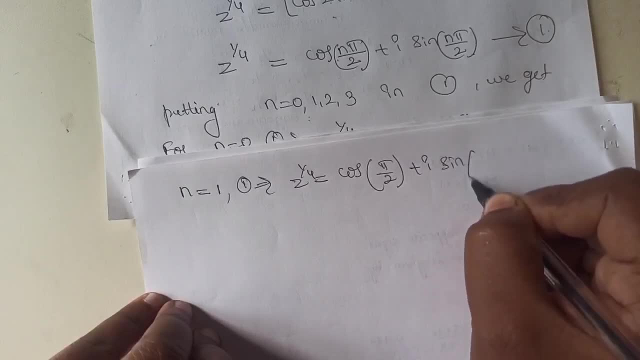 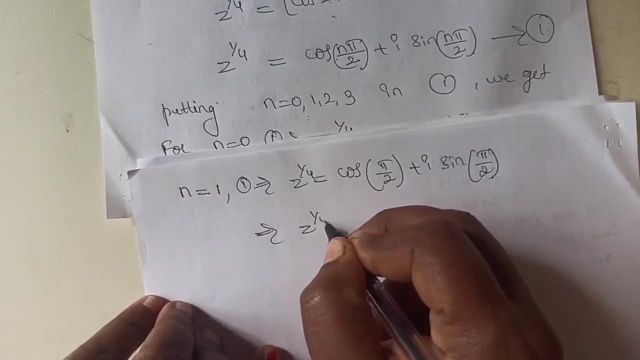 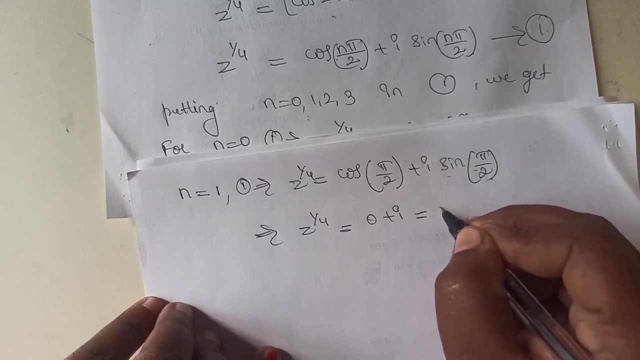 plus i sin pi by 2.. Now simplifying this one, we get z power 1 by 4, cos of pi by 2 is 0, plus i sin pi by 2 is equals to 1.. We get it is equals to 1.. So thus: 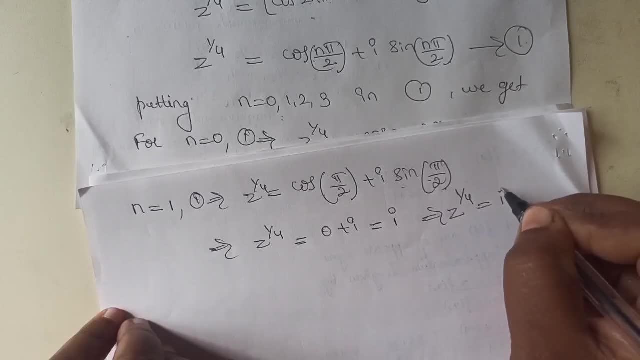 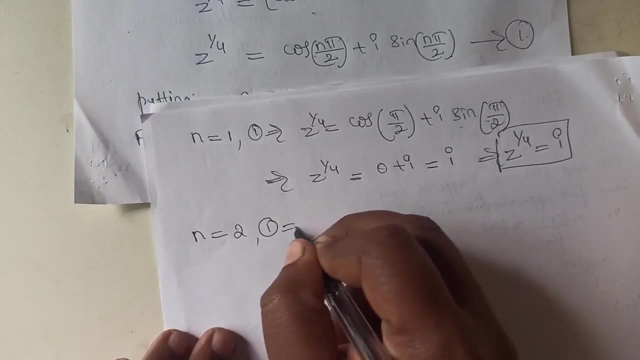 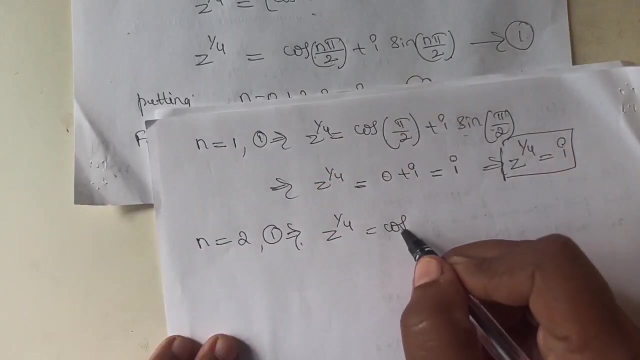 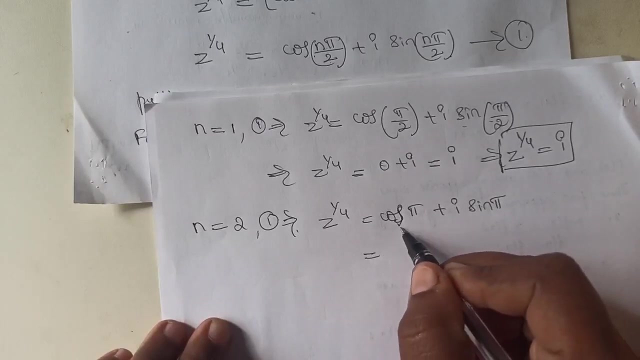 the second root is: i Okay For n equals to 2, equation 1 implies z power 1 by 4, cos of 2, pi by 2.. That is, we get cos pi plus. i sin pi. Now cos of pi is equals to minus 1. plus i sin pi by 2.. So that is, we get cos of pi plus i sin pi by 2.. So that is, we get cos pi plus i sin pi by 2.. Thus i sine pi is equal to 0.. 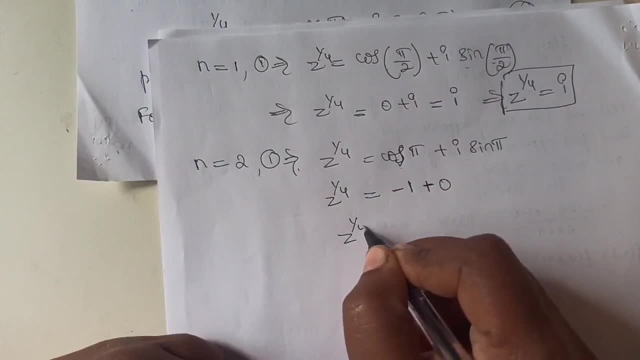 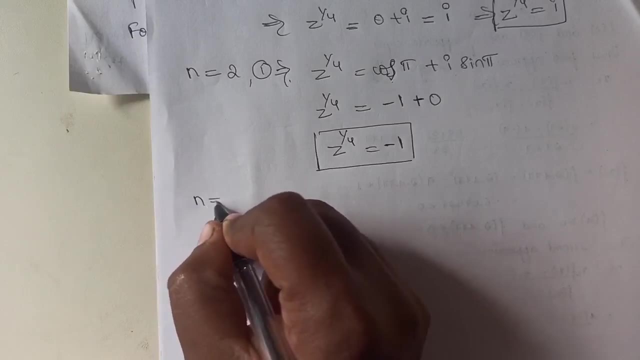 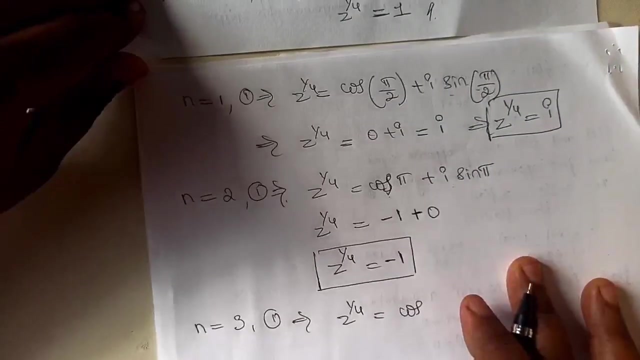 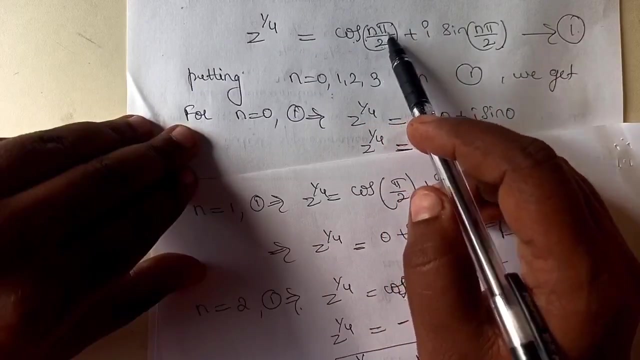 Thus the third root is minus 1.. Next, for n equals to 3, equation 1 implies that z power 1 by 4.. For cos of substituting n equals to 3 in equation 1, we get cos 3 pi by 2 plus i sine 3 pi by 2.. 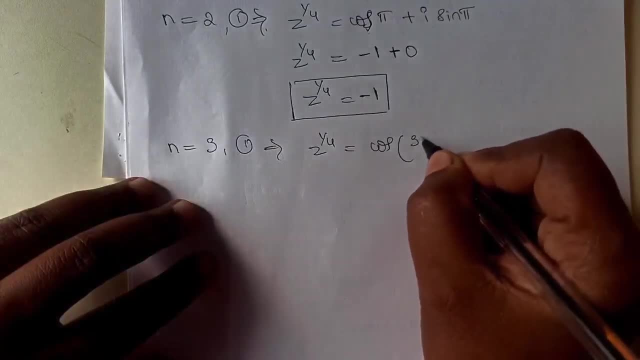 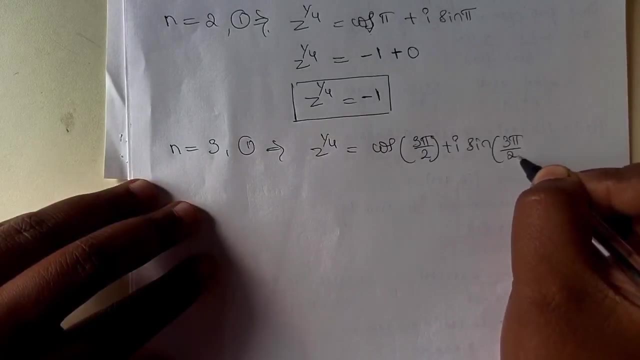 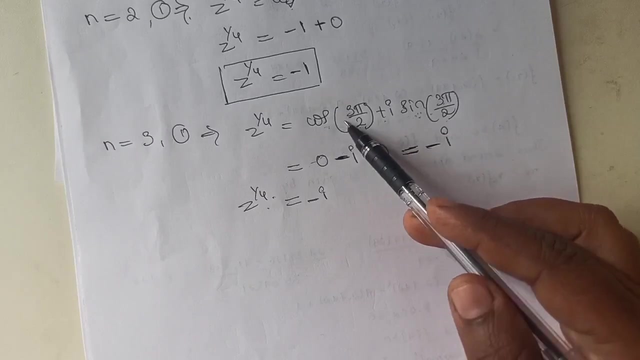 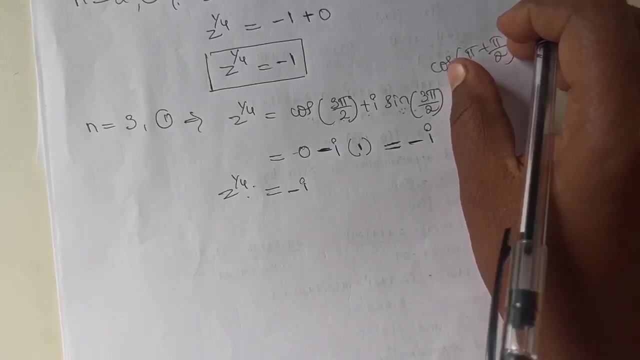 So that is, we get cos 3 pi by 2 plus i sine 3 pi by 2.. This cos of 3 pi by 2 can be written as This cos of pi plus pi by 2.. So cos of 180 plus theta lies in the third quadrant. 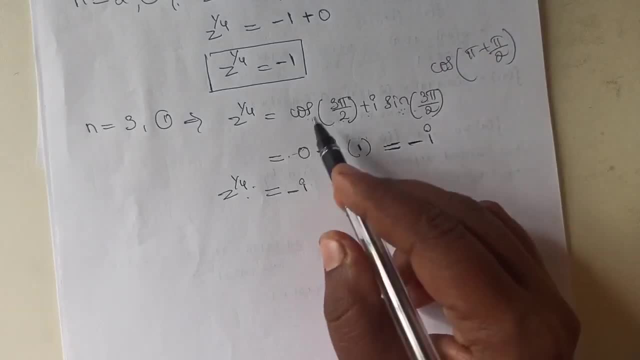 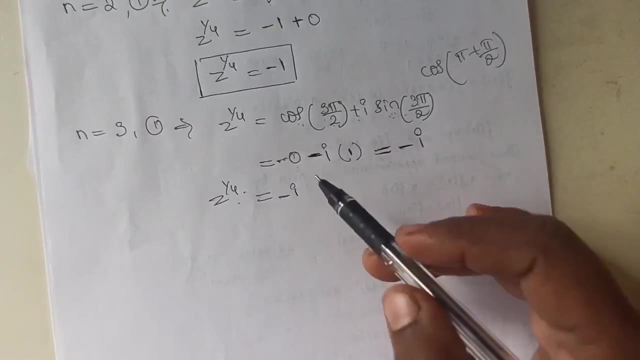 In the third quadrant, cos is negative. Therefore it is negative cos pi by 2.. But cos of pi by 2 is equal to 0. So this one negative of 0 or it simply it is 0. So similarly this can be written as sine of pi plus pi by 2.. 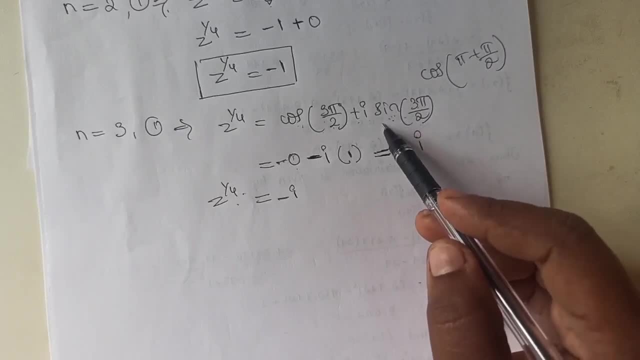 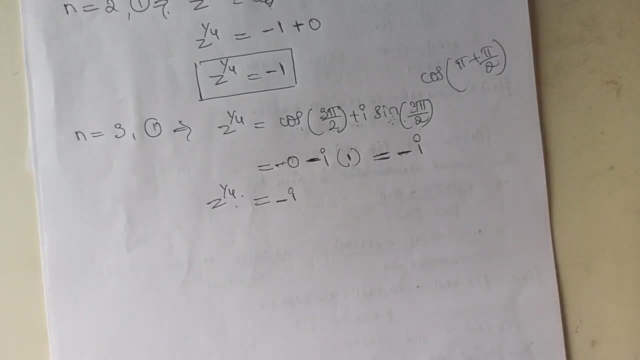 So again, it lies in the third quadrant. In the third quadrant, sine also negative, Therefore negative. So it is negative. cos pi by 2: i, as it is sine of pi by 2, is equal to 1. So therefore it is equal to minus i. 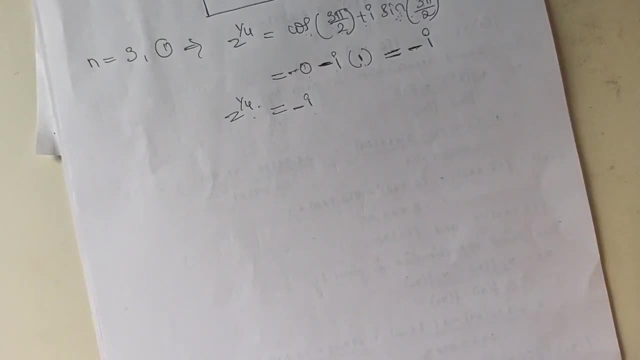 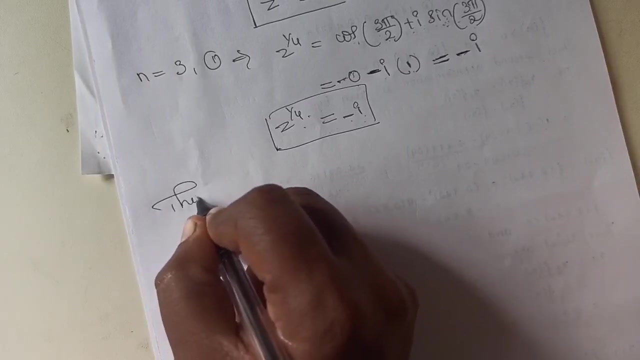 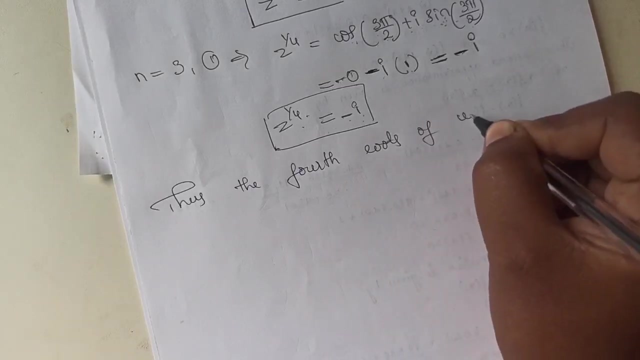 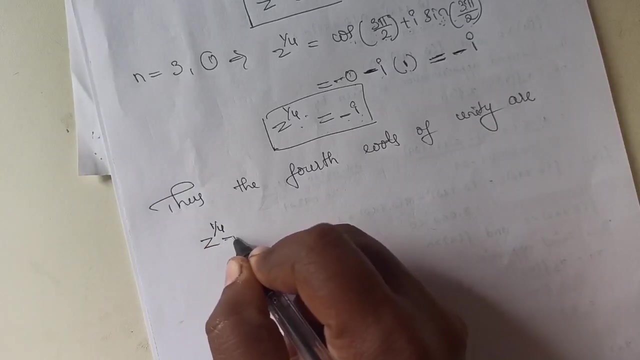 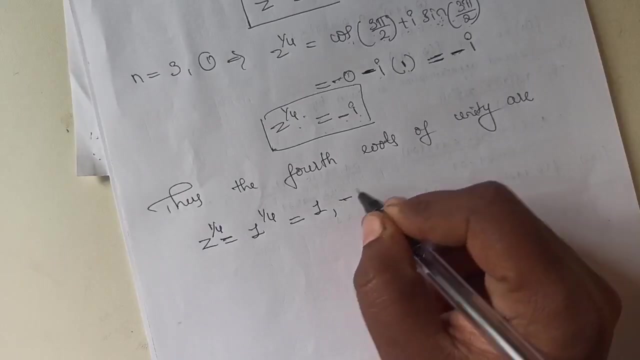 So z power 1 by 4 is equal to minus i. Okay, So therefore the fifth root, fourth root, is minus i. Thus the four roots of unity are z equals z power 1 by 2. So z power 1 by 4, which is equal to 1, power 1 by 4 are 1 minus 1.. 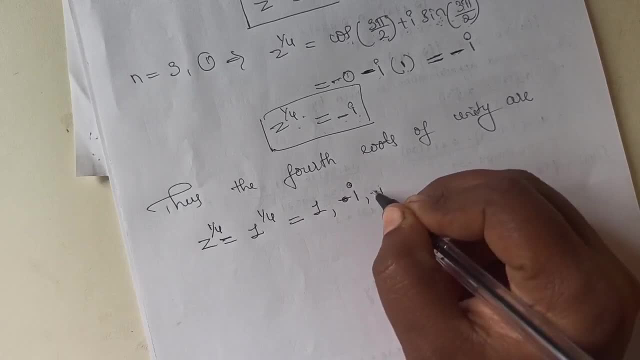 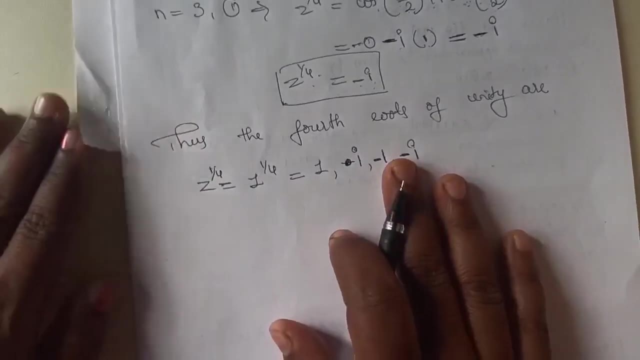 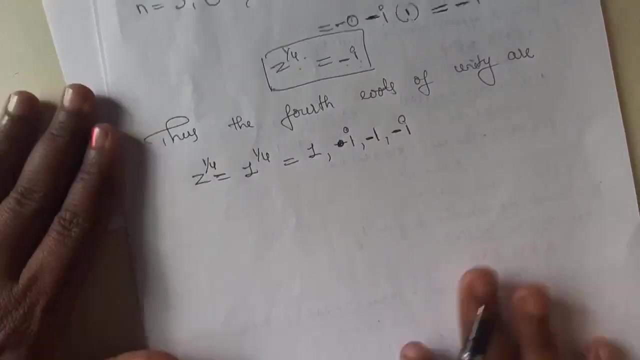 So 1 or 1 i minus 1 and minus i. So these are the fourth roots of unity. Okay, So these are the fourth roots of unity. Next, we want to represent it in the arrogant plane. For that we draw a circle. 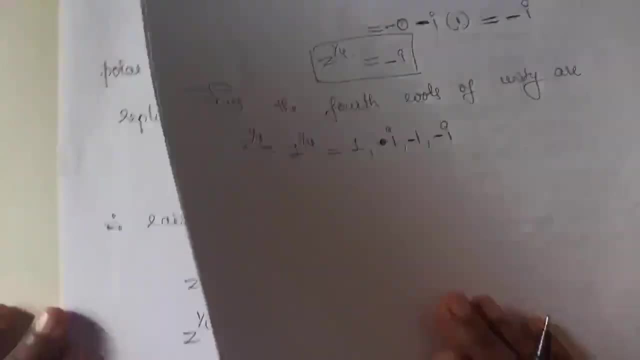 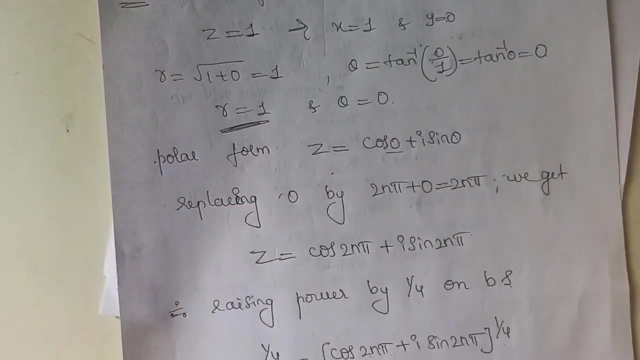 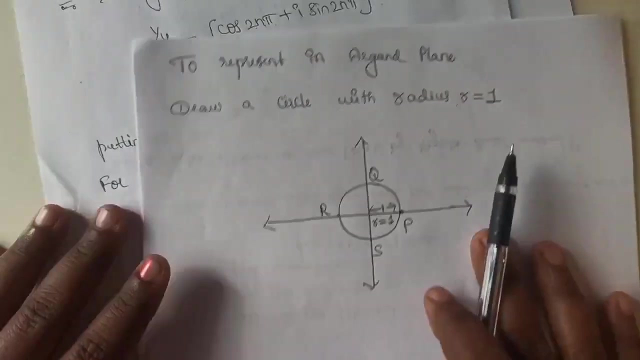 With the radius r equals to 1.. Since here we got, r, value is equals to 1.. Therefore, we draw a circle: r equals to 1.. Okay, Now we draw a circle with radius r equals to 1.. So that is. 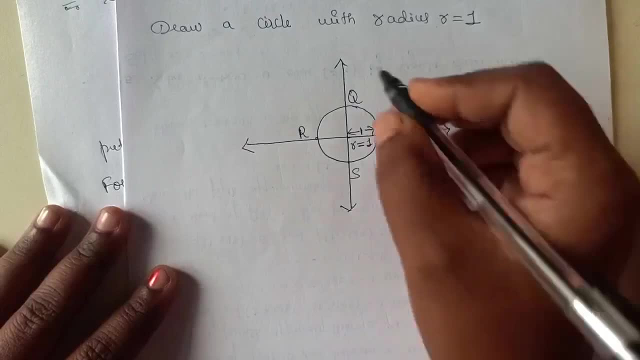 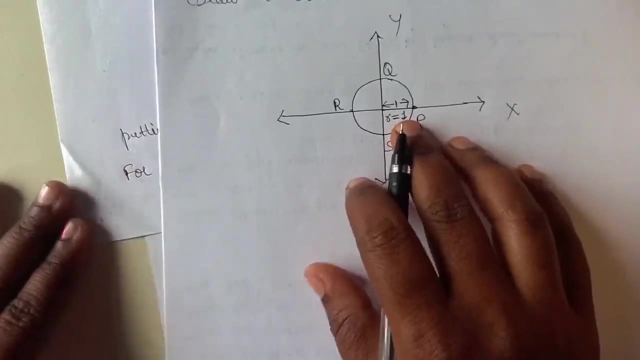 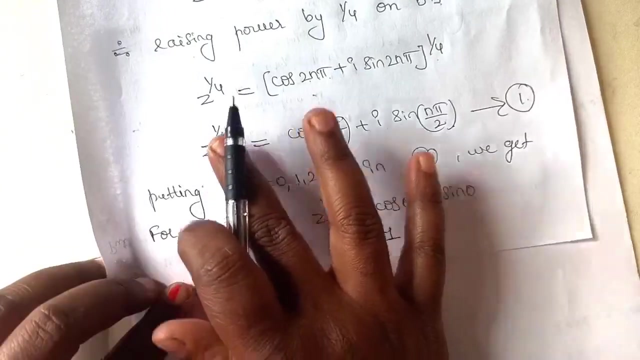 So this is the arrogant plane That is x axis. This is x axis and y axis. Okay, Here we have drawn a circle of radius 1.. Okay, So this is the circle Now. next. Next, we substitute: n equals to 0,, 1,, 2,, 3 in the z power 1 by 4 argument of the z power 1 by 4.. 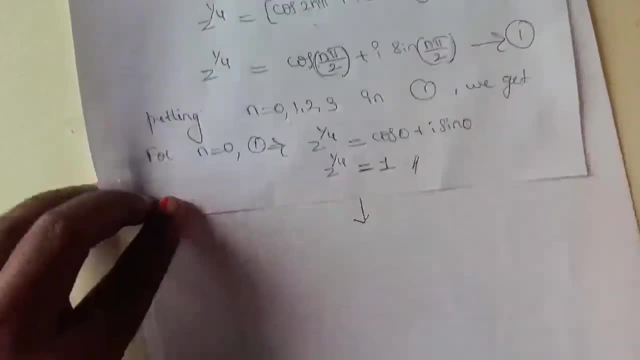 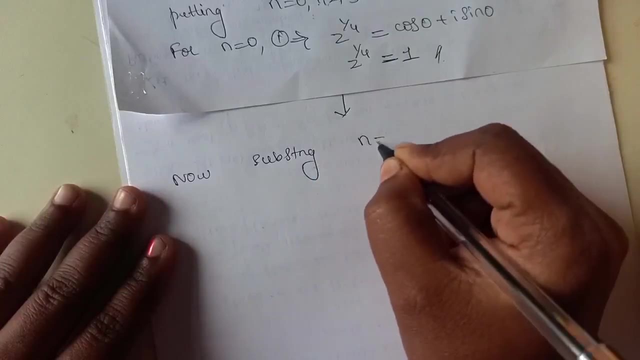 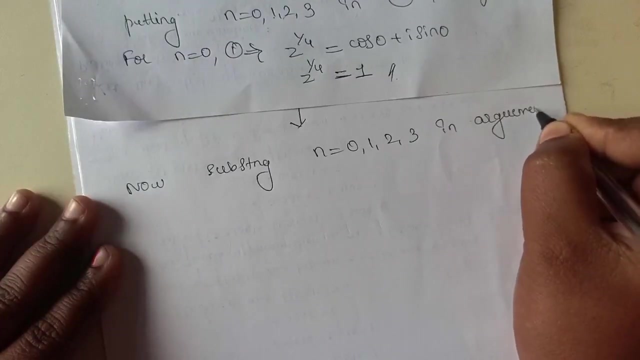 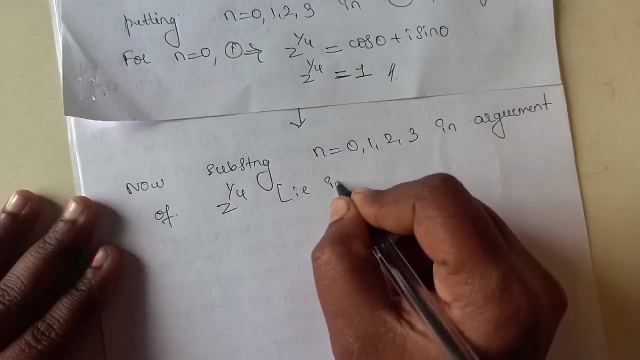 That is in this argument n pi by 2.. Okay, So now substituting n equals to 0,, 1,, 2, 3 in argument of z power 1 by 4.. So that is in equation 1.. 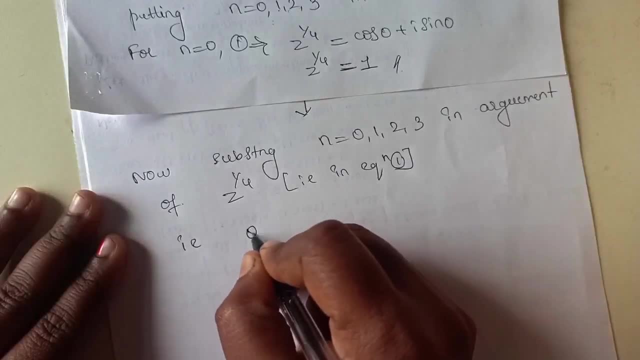 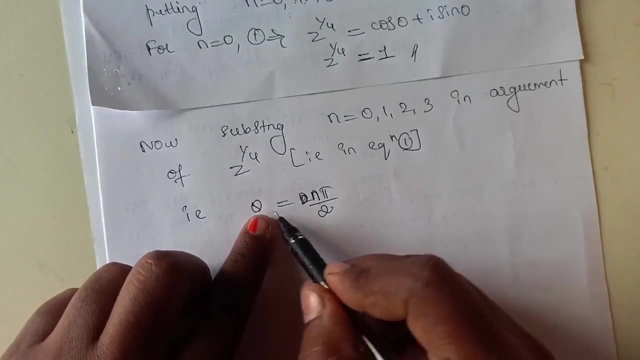 So that is, theta is equals to 2n. Sorry, here Theta is equals to n pi by 2.. So we substitute: n equals to 0,, 1,, 2,, 3 in theta is equals to n pi by 2.. 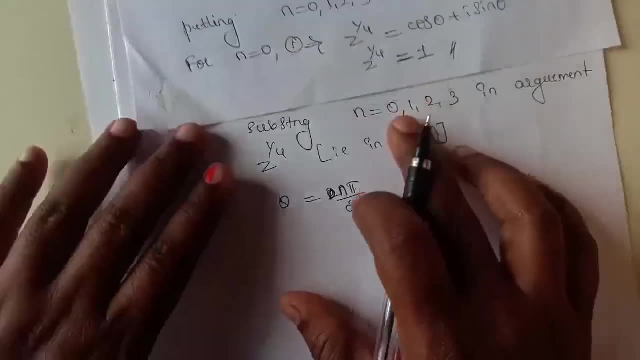 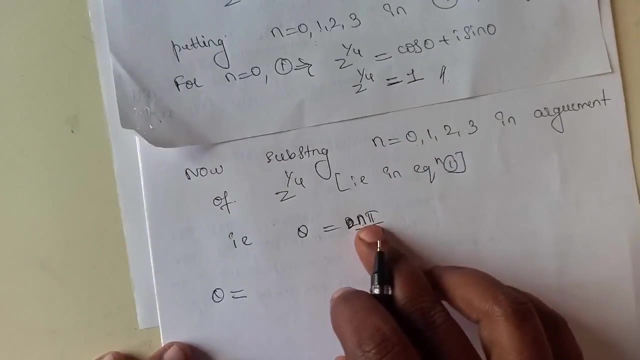 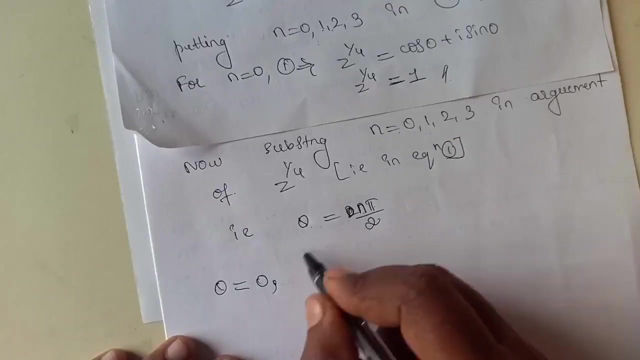 Okay. So substituting n is equals to 0, we get. So theta is equals to: Okay. So now, substituting n equals to 0, we get 0.. And substituting n equals to 1, we get. theta is equals to n pi by 2.. 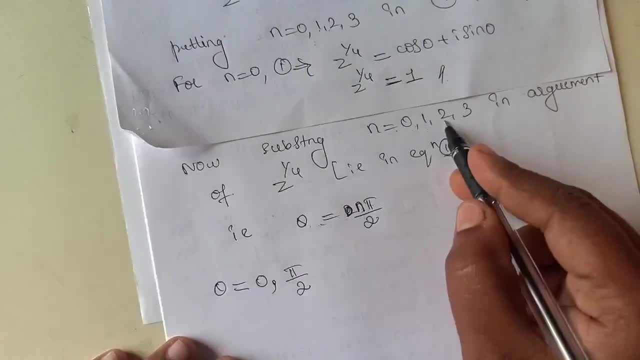 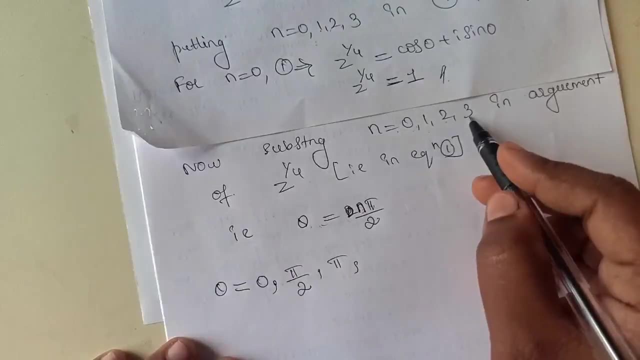 That is pi by 2.. Next substitute 2, 2 pi by 2. So 2,: 2 get cancels, We get pi. And substituting n equals to 3, we get 3 pi by 2.. 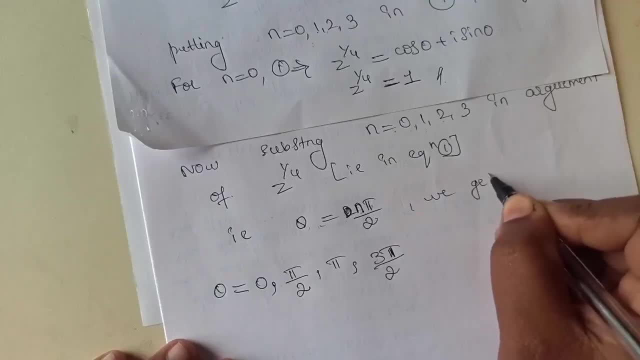 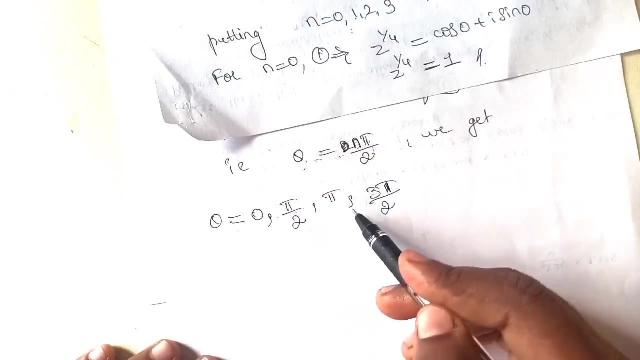 Okay, Okay, So now substituting. So now substituting: n equals to 0,, 1,, 2, 3 in theta is equals to n pi by 2, we get: theta is equals to 0, pi by 2, pi 3 pi by 2.. 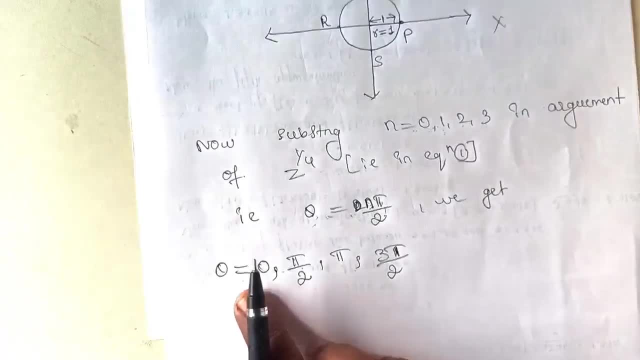 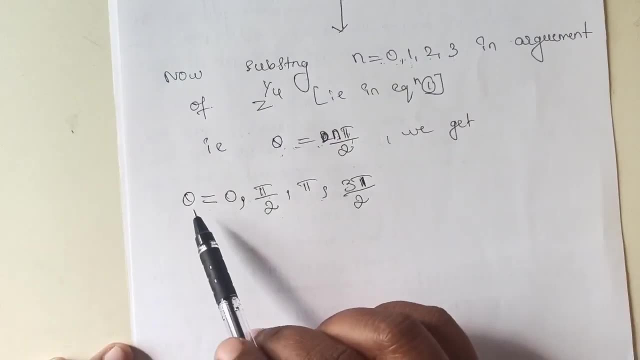 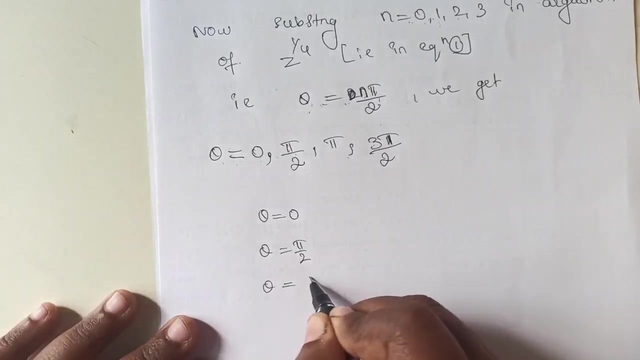 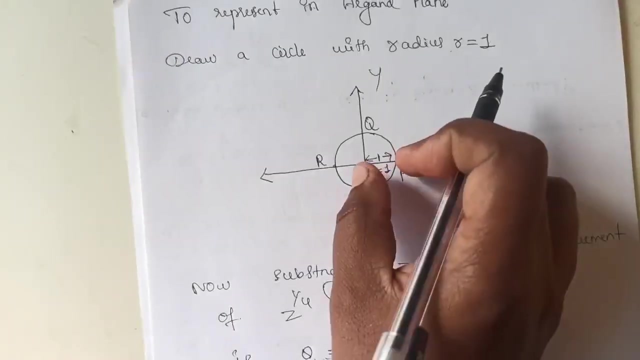 Okay, Now we draw the lines: theta is equals to 0 and theta is equals to pi by 2, theta equals to pi and theta is equals to 3 pi by 2.. So you can observe that Theta is equals to 0 is the x-axis itself. 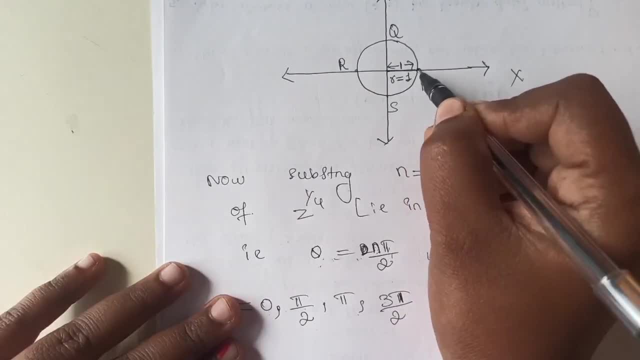 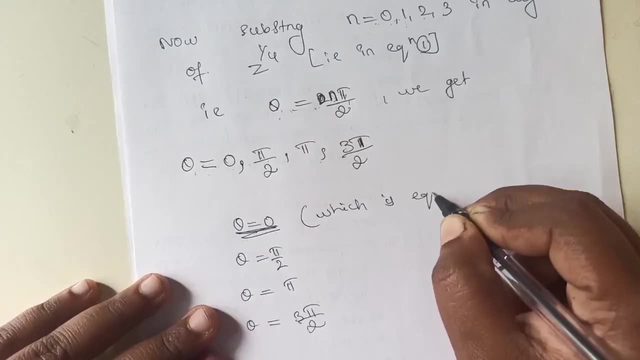 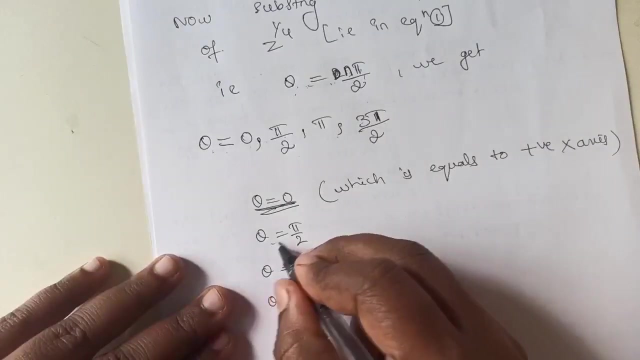 Okay, We draw. theta is equals to 0. Therefore it lies in the x-axis only, So which is equals to positive x-axis. Okay Now theta is equals to pi by 2.. Definitely, this will be the positive y-axis. 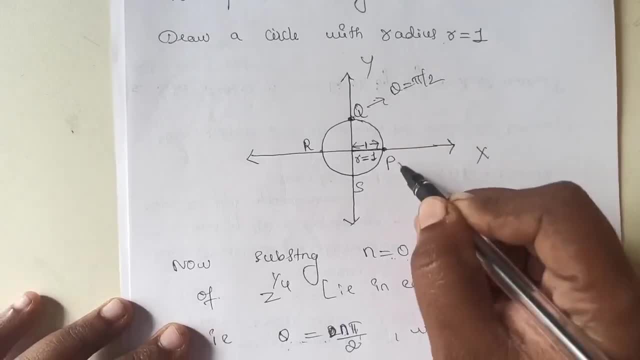 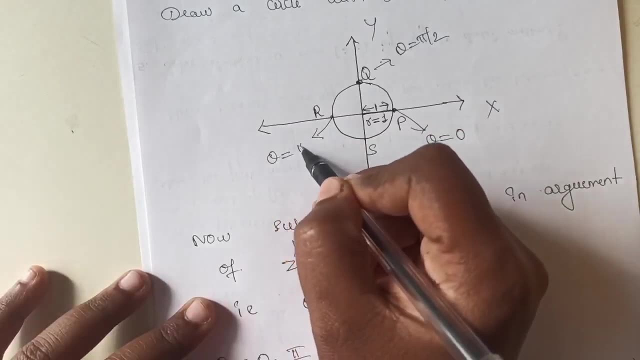 So this is: theta is equals to pi by 2.. So here This point is: theta is equals to 0. Definitely this will be: theta is equals to pi. and this is theta is equals to 3 pi by 2.. 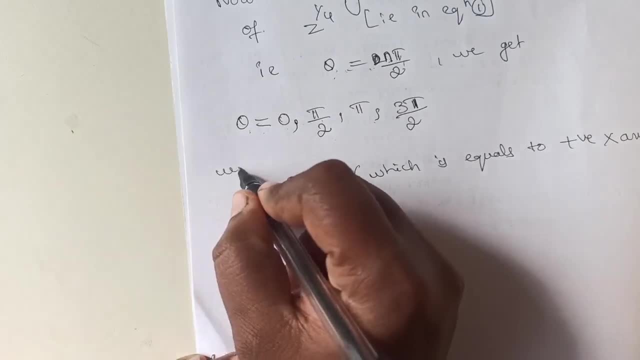 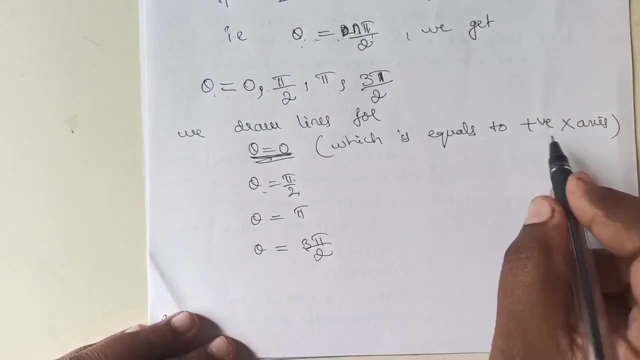 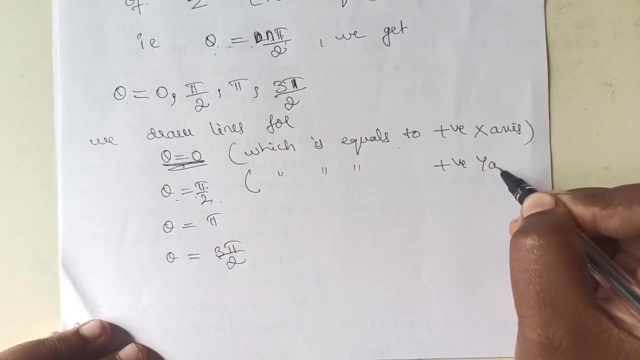 Okay, So on drawing. So that is, we draw lines, for theta is equals to 0, which is equals to positive x-axis. So next, theta is equals to pi by 2, equals to the positive y-axis. Next, this is same. 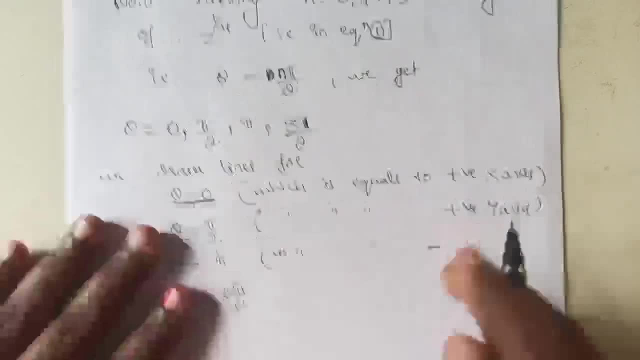 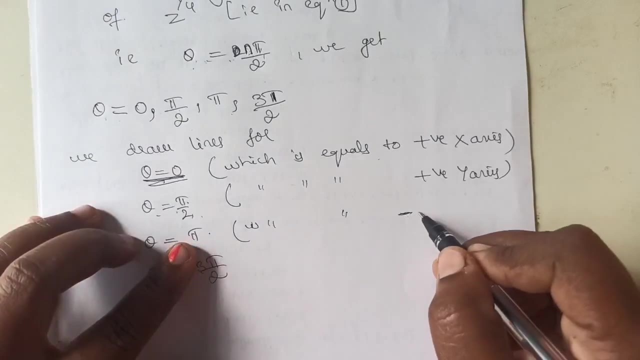 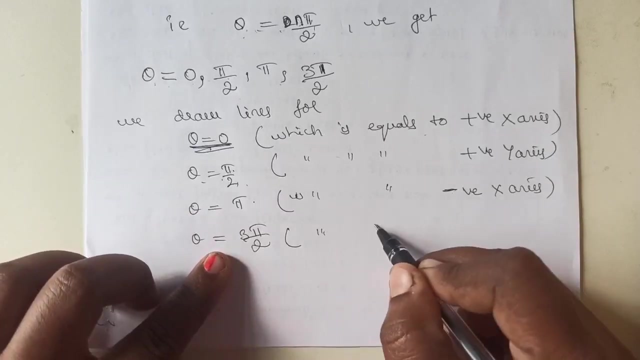 It is equals to. So this theta is equals to pi. Pi means 180.. This is equals to negative x-axis. So it is equals to negative x-axis, And definitely So. this will be equals to negative y-axis. 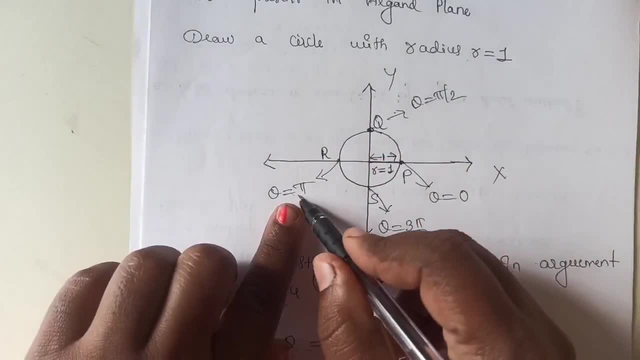 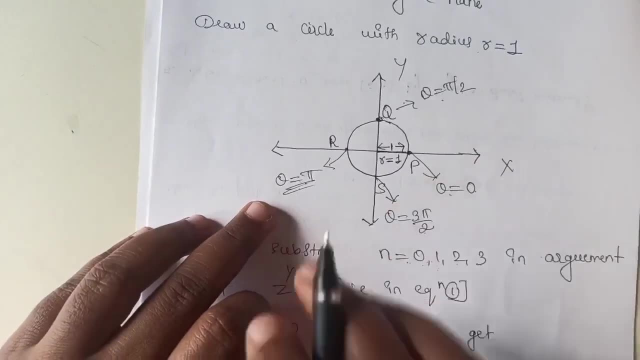 Okay, Now got this one. This is: theta is equals to 0.. Theta is equals to 3.. Pi by 2. Theta is equals to 0.. Theta is equals to pi by 2.. So sorry, This is: theta is equals to pi. 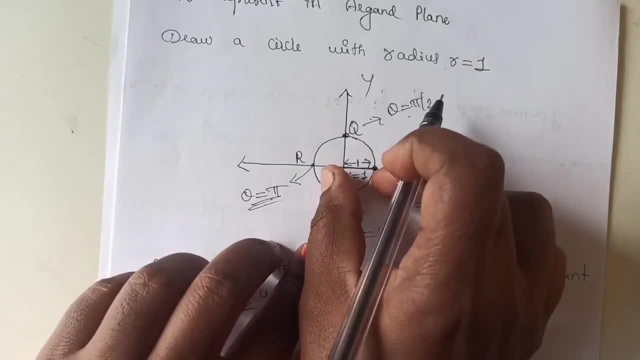 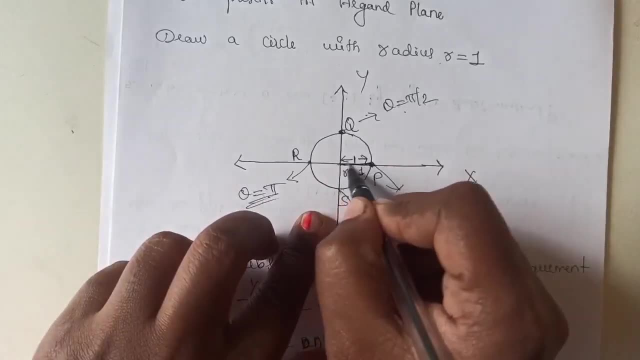 Okay, So you can observe that Here r is equals to 1. This x-distance is equals to 1. But this y-distance here in this line, For this line. Okay, We write the points For this line p. 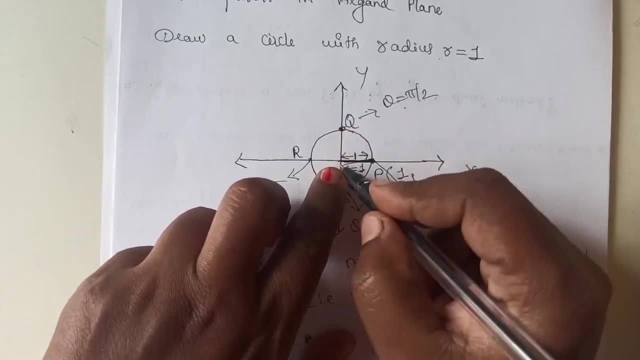 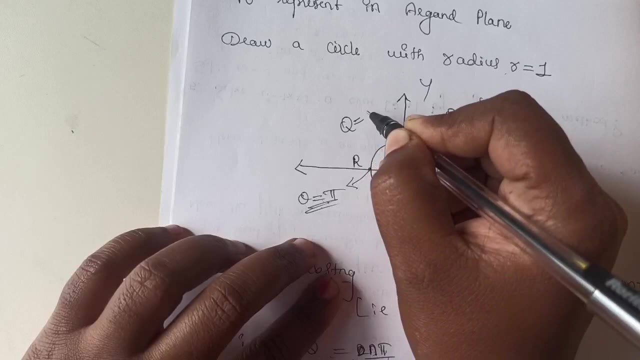 x-axis equals to 1.. But y-axis, here it is equals to 0.. Okay, For this point q. So this point, This distance is again 1.. So this is: y-distance equals to 1.. But x-distance is 0.. 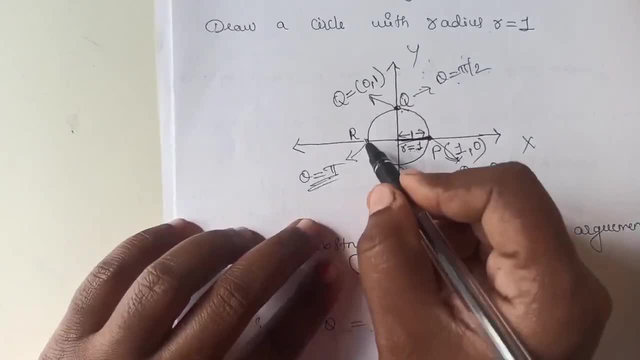 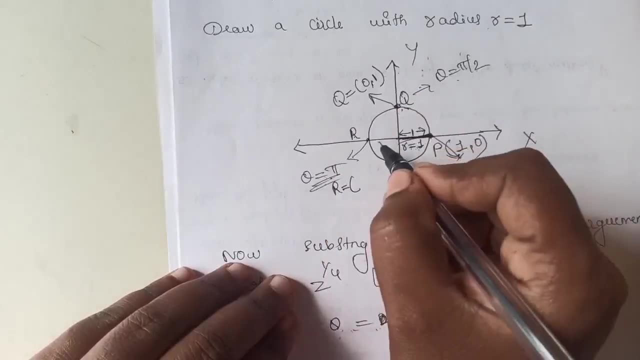 Therefore we can write it as 0, 1.. Similarly, for this one r is equals to, So this is negative of x-axis. So here this will be minus 1.. So minus 1, y-distance is 0.. 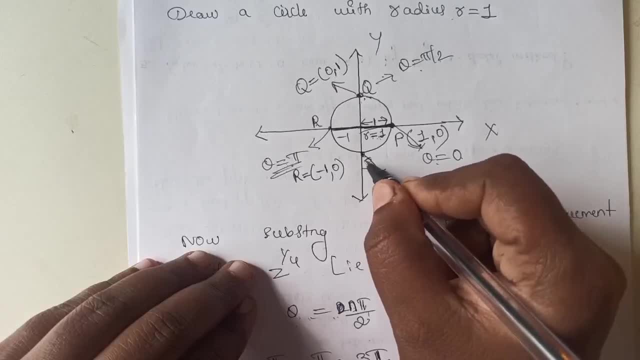 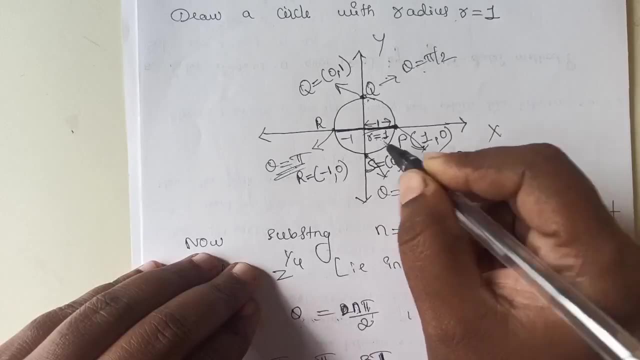 For this point s is equals to. It is negative of y-axis, But y-distance is 0. So this is negative of y-axis, So x-axis is 0.. Therefore x-axis is 0. But y-axis is minus 1.. 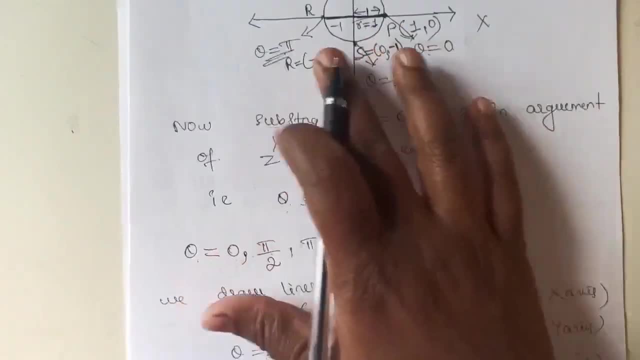 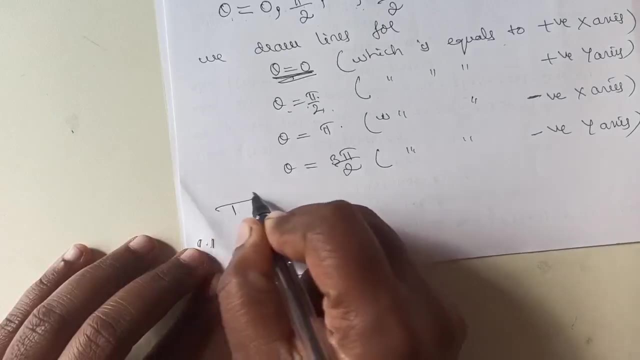 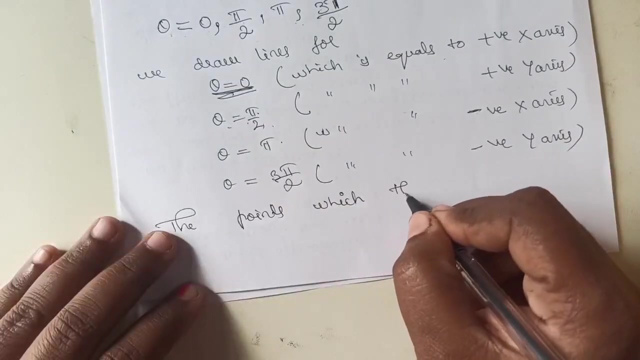 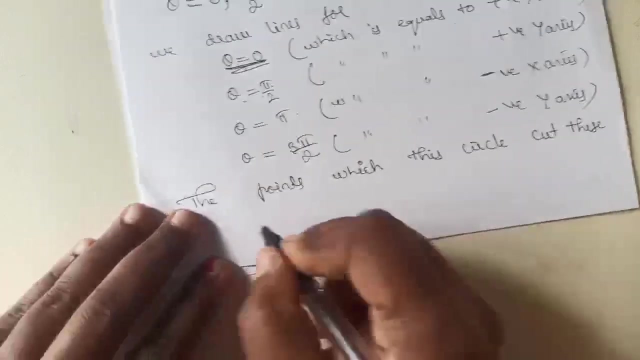 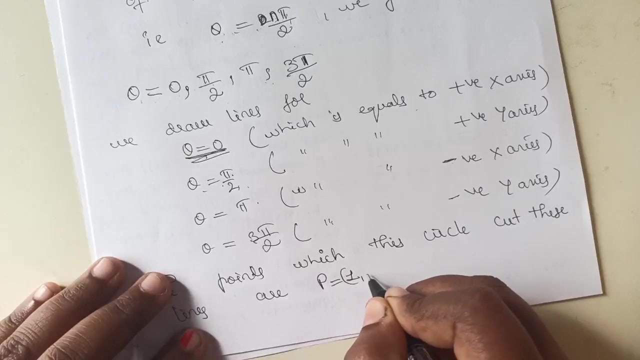 So therefore, we can observe that all these points represent 5th roots of unity. Okay, That is the point which this circle cut these lines. The first point is: p equals to 1, 0.. Second one: q equals to 0, 1.. 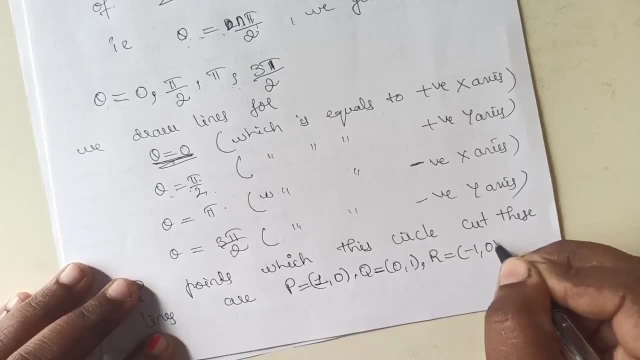 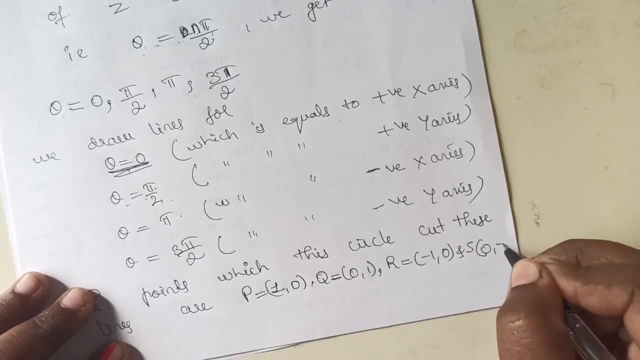 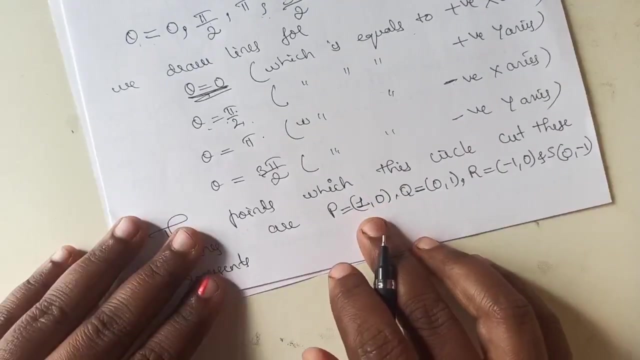 r equals to minus 1, 0. And theta s is equals to 0, minus 1.. So these points represent And 4th roots of unity. That is, if you transform this into complex number, you will get 1 plus 0i. 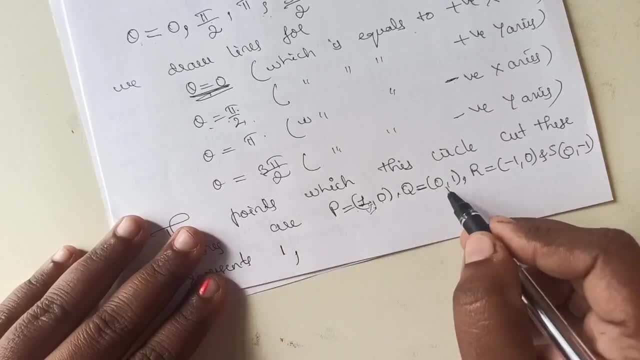 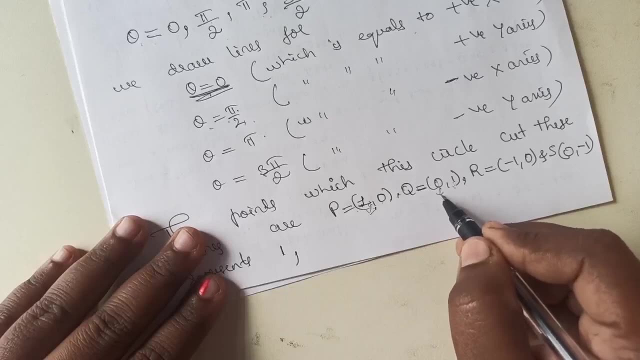 That will be 1 only, So transforming into complex form: 0 plus 1i. Okay, You add i: Okay, So this is x-value And this will be the y-value, x plus iy. Okay.